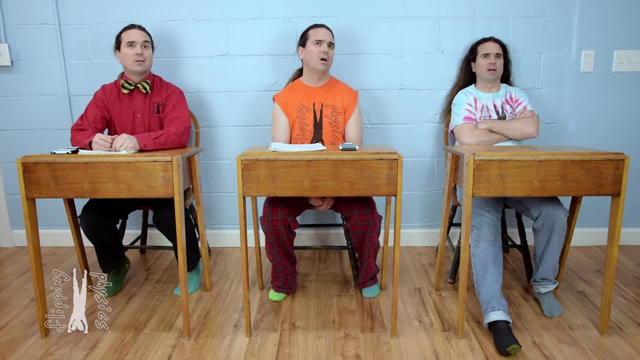 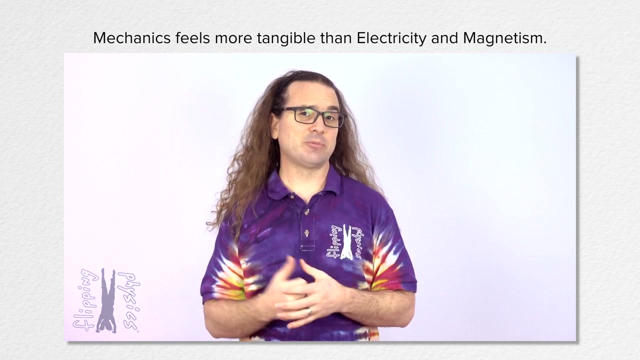 Uh no, He said: begin reviewing. I think we are only reviewing electric charges and fields today. Okay, good, All of AP Physics C, Electricity and Magnetism would be a lot. Mechanics tends to feel a lot more tangible to my students than electricity and magnetism. 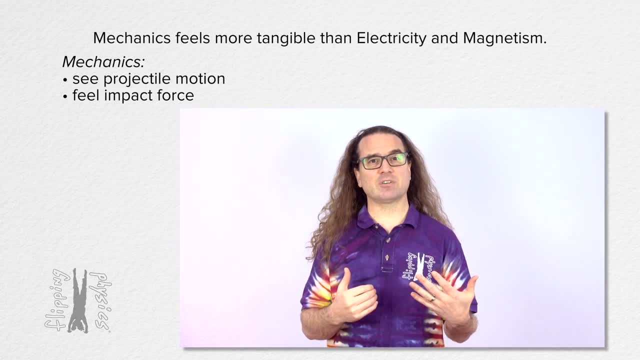 You can see projectile motion. You can feel an impact force when an object runs into you. You can feel rotational inertia change as you change the mass distribution of an object. I do not get the gist of it. I think I am the only one who is not done with electrical. 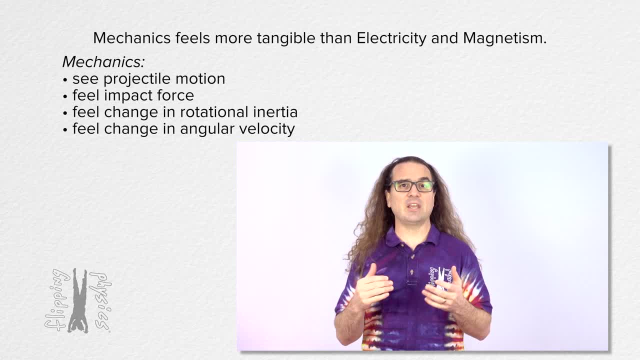 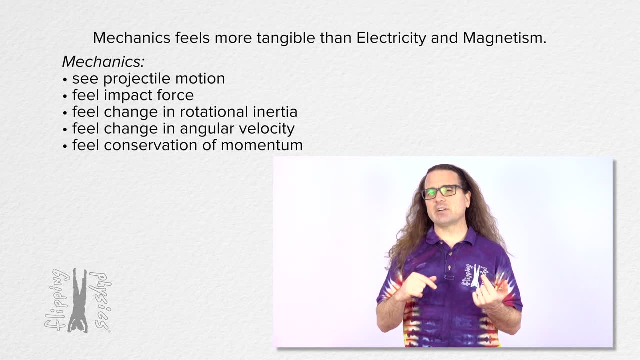 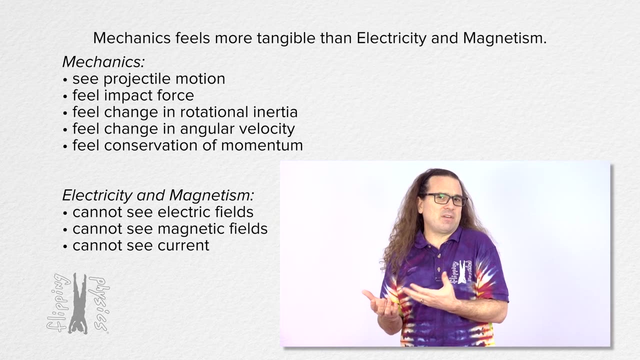 object. You can feel a change in angular velocity as you change your rotational inertia. while spinning You can feel conservation of linear momentum when you catch something. However, it is much more difficult to visualize electric and magnetic fields. You cannot really see current moving through wires. You have to visualize Gaussian surfaces And you can actually see. 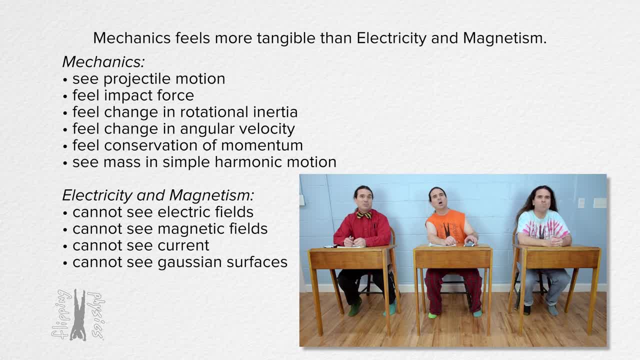 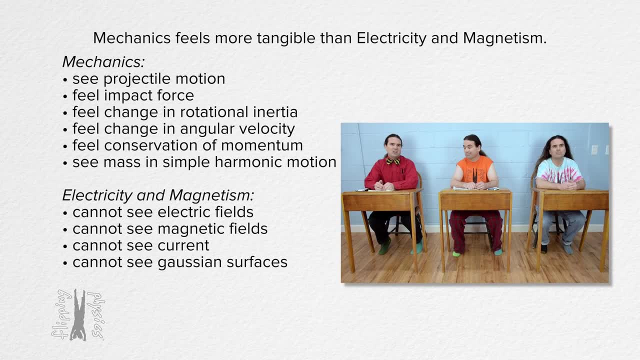 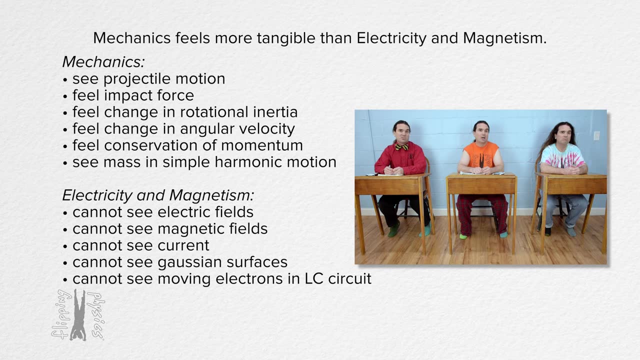 the mass in an oscillating mass-spring system moving back and forth in simple harmonic motion, which makes it so you can visualize the kinetic and elastic potential energies. However, in an inductor-capacitor circuit, you cannot see the moving electrons causing the energy to be stored. 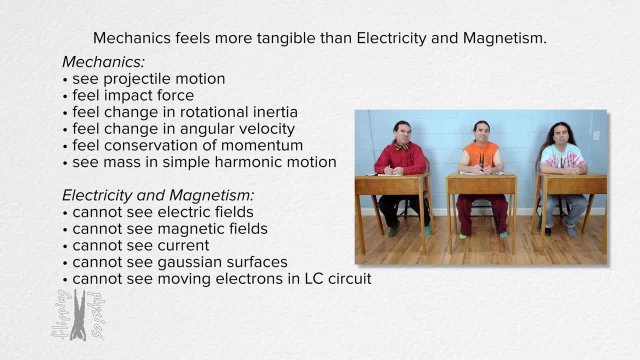 in the electric field in the capacitor and the magnetic field in the inductor. Yeah, mechanics is a lot more tangible than electricity and magnetism. Sure, Exactly This makes it so typically my students tend to struggle a bit more at the beginning to 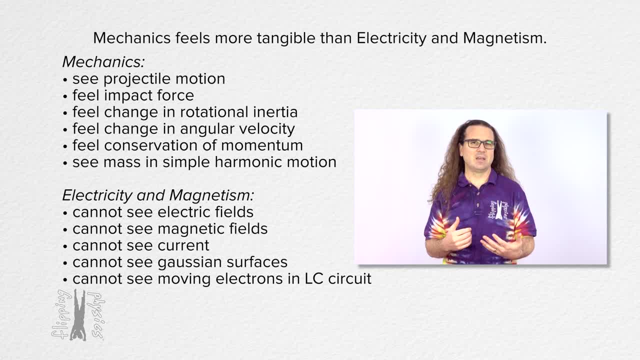 understand electricity and magnetism than they do mechanics. I do want to make it clear, though, that after students have spent time learning and visualizing electricity and magnetism concepts, typically they feel that these two curricula end up being about the same level of difficulty. Electricity and magnetism does take a bit of 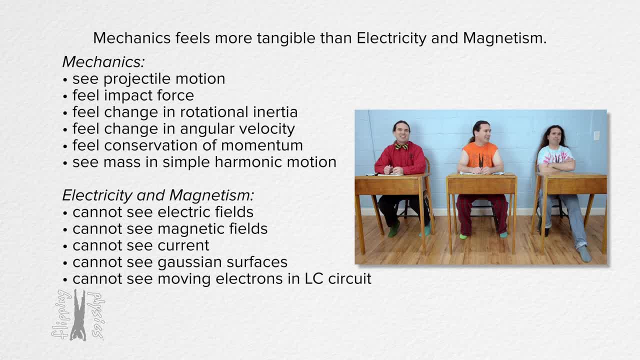 time to get used to, though. Yeah, I agree with that Totally. I love electricity and magnetism, But do you love it more than mechanics? I love them both, Of course. Alright, here we go. Billy, please tell me about electric charge. 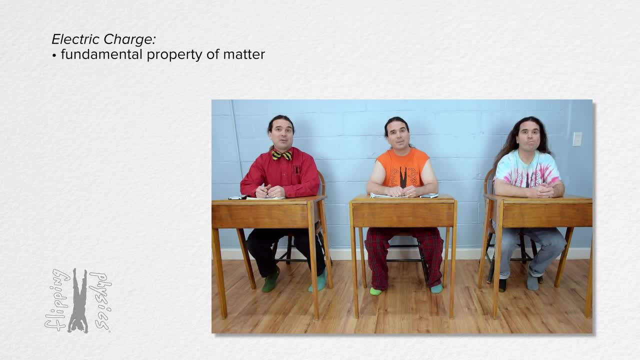 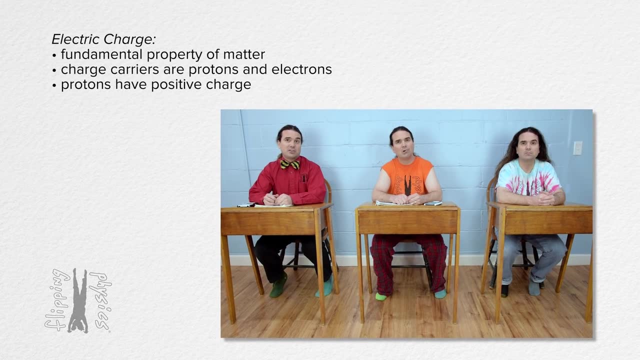 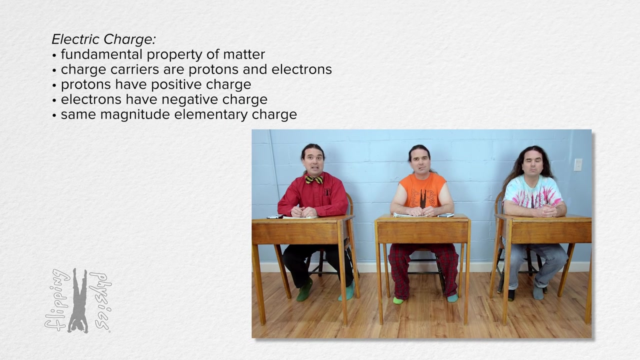 Okay, Electric charge is a fundamental property of all matter. The charge carriers are protons and electrons, where protons have a positive charge and electrons have a negative charge. Both protons and electrons have the same magnitude charge, called the elementary charge, The symbol. 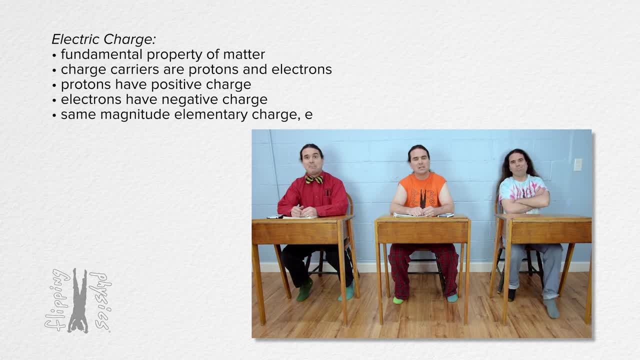 for the elementary charge is a lowercase e and it has a magnitude of 1.60 times 10 to the negative 19 coulombs. That is the elementary charge because it is the absolute value of the charge on both a proton and an electron. But again, the proton has a positive charge and an electron has a negative. 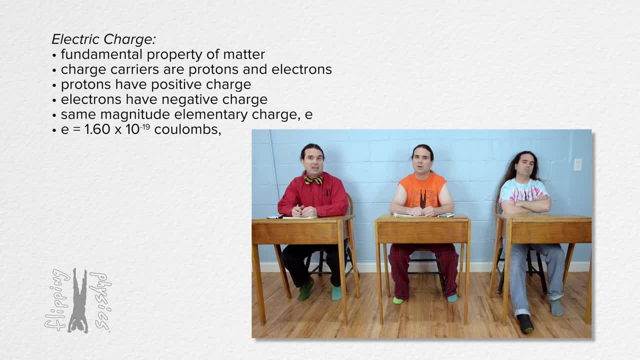 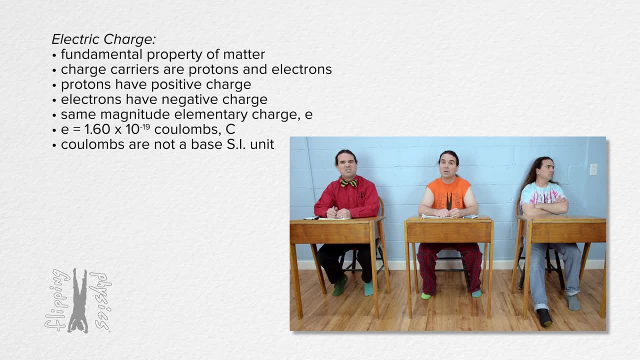 charge. The symbol for coulombs is a capital C. Coulombs are not a base SI unit. I always found it weird that amperes are a base SI unit instead of coulombs, but they are Okay. Charge is a scalar quantity. Charge is quantized, In other words, it comes in discrete. 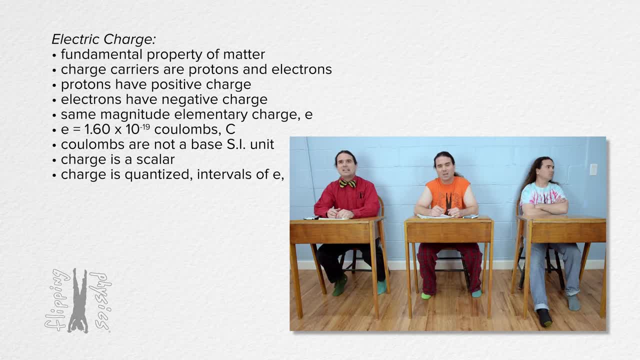 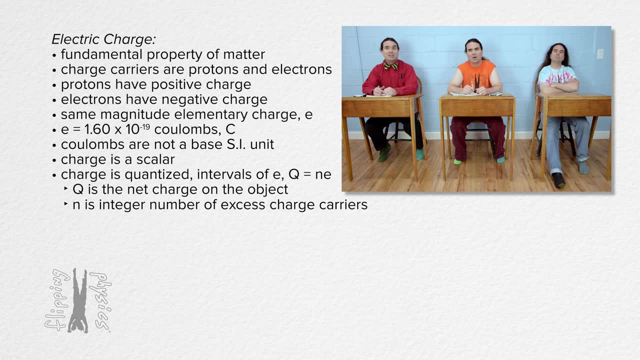 quantities and intervals of the elementary charge. That is actually an equation. The net charge on an object, uppercase q, equals lowercase n the integer number of excess protons, or positive or negative charges on the object times lowercase e the elementary charge, And n is either positive 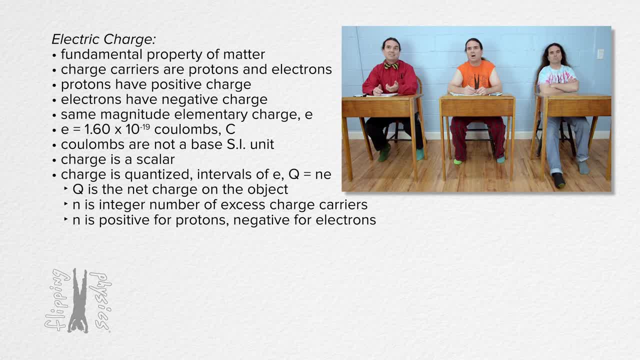 or negative. depending on whether the excess charges are positive or negative, Quantization of charge means an object will never have, for example, a charge of positive 2.1 times 10 to the negative 19 coulombs, because that is not an integer multiple of 1.60 times 10 to the negative 19. 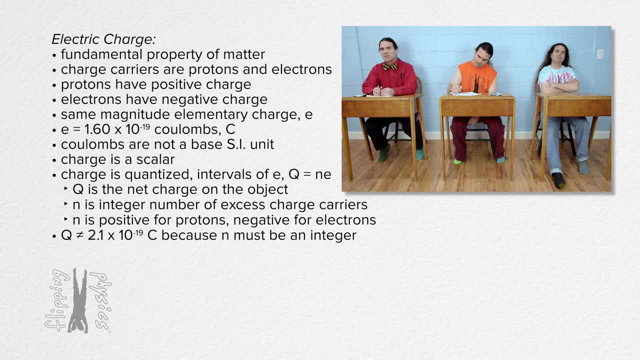 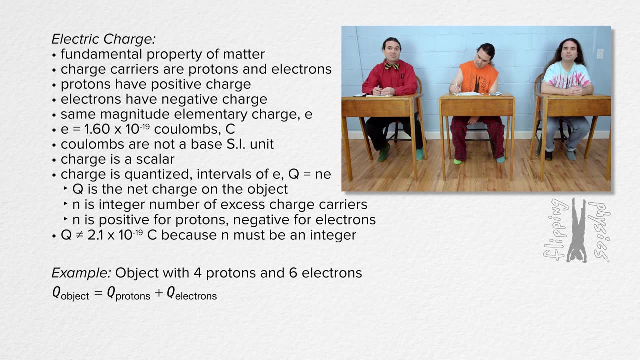 coulombs the elementary charge. The electric charge on an object is determined by the total number of charge carriers contained in the object. For example, the electric charge on an object with 6 electrons equals the charge on the protons plus the charge on the electrons, or positive 4 times. 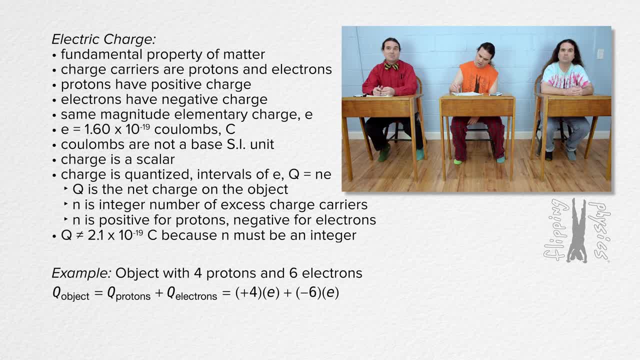 the elementary charge plus negative 6 times the elementary charge, which is negative 2 times the elementary charge. In other words, the net charge on this object is the same as if it contained only 2 electrons. It equals negative 2, the total number of excess electrons times 1.60 times. 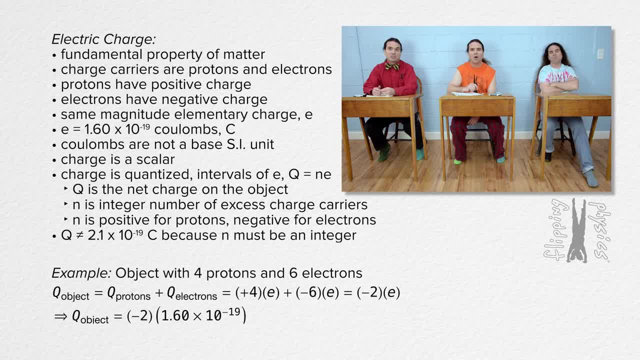 10 to the negative 19,, which is the absolute value of the charge on an electron or the elementary charge, and that works out to be negative 3.20 times 10 to the negative 19 coulombs. Many objects we work with will be considered to be point charges, even if they are made up of: 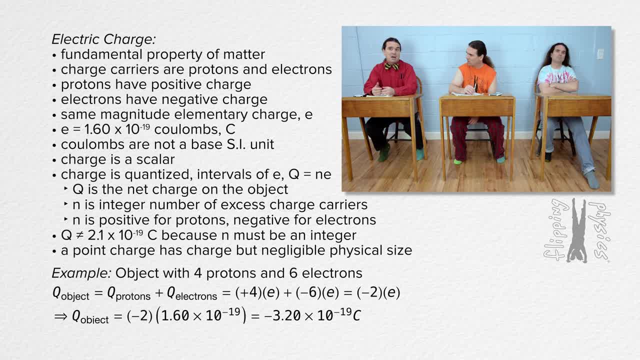 many charge carriers, and a point charge is a model of a charge where the physical size of the charge or the charged system is small enough to be considered to be negligible. That is all I can think of right now. You really do love this stuff. 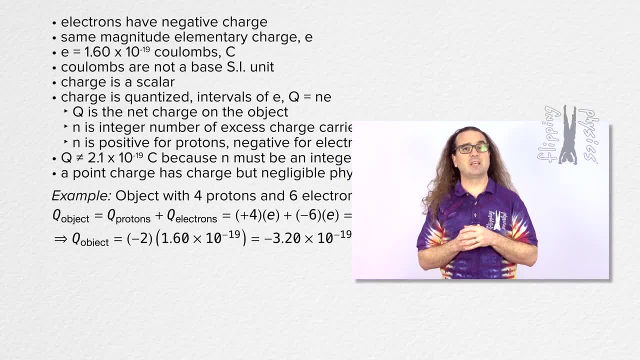 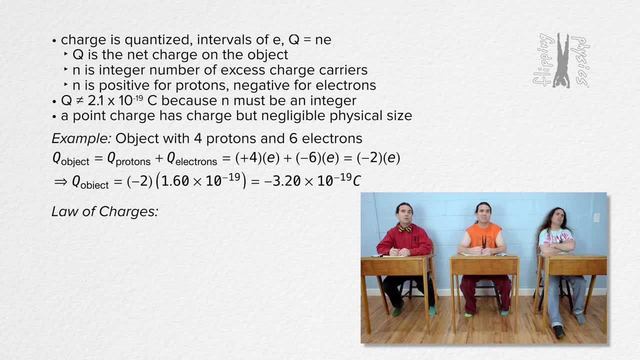 Yeah, Yeah, Thank you very much, Billy. Bobby, tell me about the Law of Charges. The Law of Charges, Well, that states that two charges with opposite trait one another and two charges with the same sign repel one another. 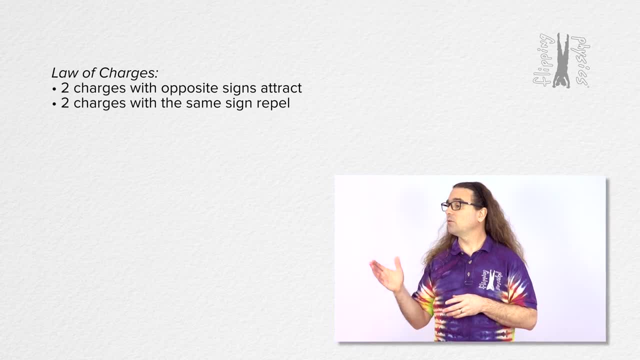 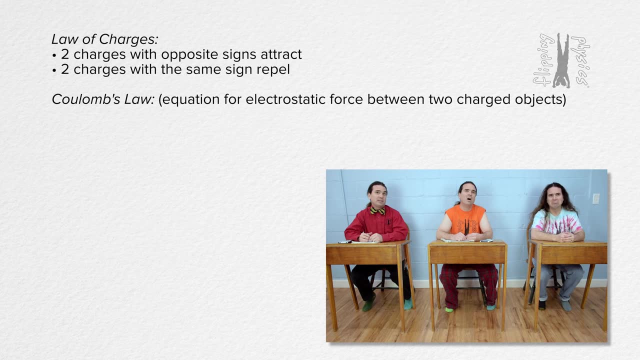 That's it. that's the Law of Charges. Correct, Bo. coulomb's law, please. Coulomb's law, It is the equation for the electrostatic force between two charged objects. Alright, yeah, I forgot that it's called Coulomb's Law. That is the electrostatic force. 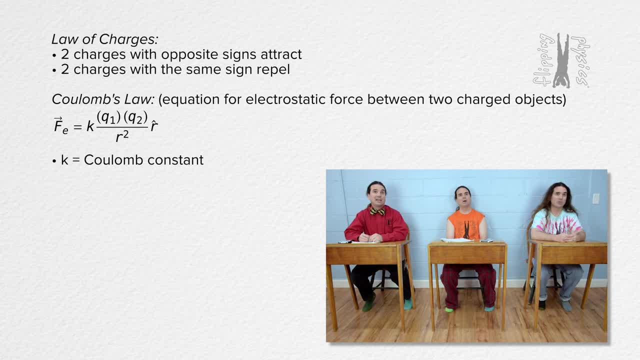 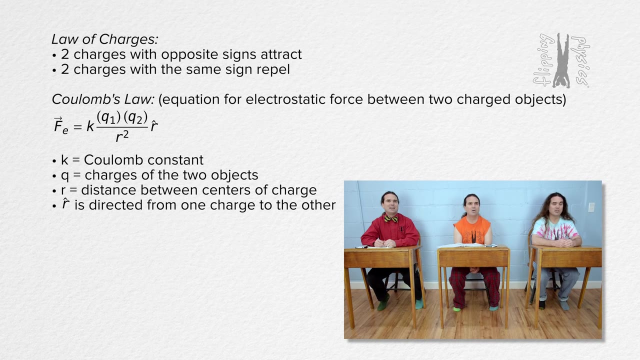 which is a vector, equals Coulomb's constant lowercase k times charge 1, times charge 2, all divided by the square of r, the distance between centers of charge of the two charges, all times unit vector r, which is directed from one charge to the other. 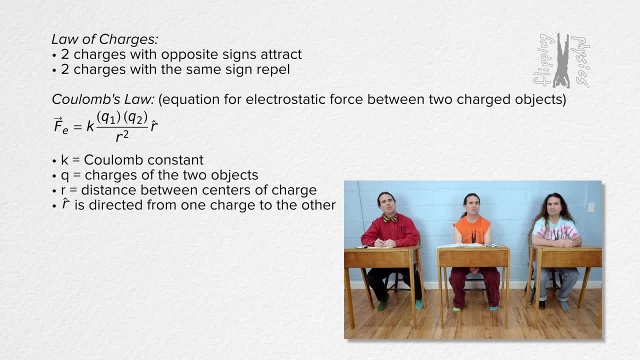 That is not the equation for Coulomb's Law. that is on the AP Physics C equation sheet. Okay, then take the absolute value of both sides and the unit vector disappears because it has a value of 1.. That is still not the equation for. 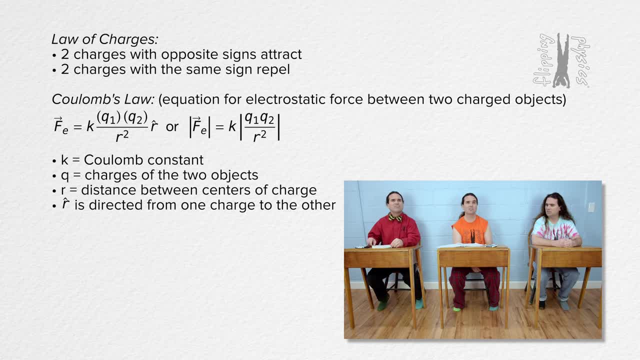 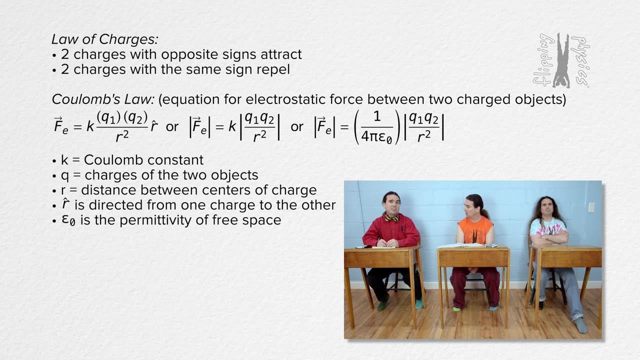 Coulomb's Law. that is on the AP Physics C equation sheet. Then what is on the equation sheet Instead of Coulomb's constant? it's 1 over the quantity 4 pi times epsilon naught. What is that? Lowercase epsilon naught stands for the permittivity of free space, and Coulomb's 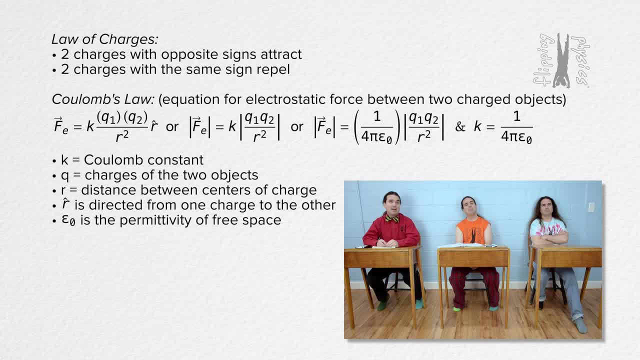 constant equals 1 divided by the quantity, 4 pi times the permittivity of free space. Yeah, Yeah, That's right. Thanks, You're welcome. But what is the permittivity of free space? Lowercase epsilon naught is the permittivity of. 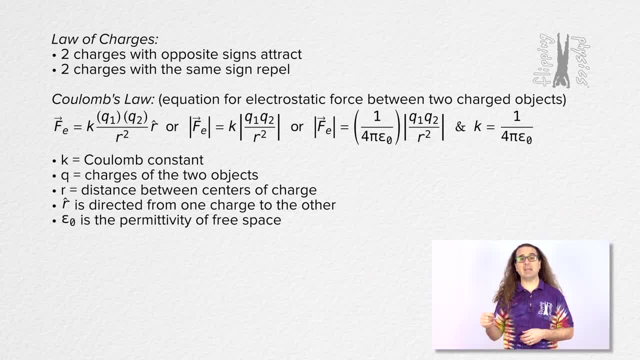 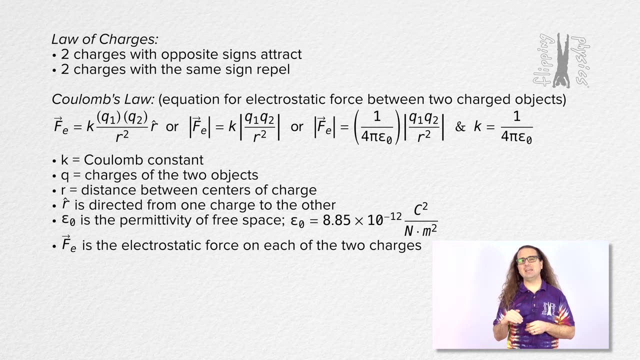 free space or vacuum permittivity, and it equals 8.85 times 10 to the negative 12 coulombs squared divided by newtons times meters squared. We will better define it when we get to capacitors and dielectrics And, to be clear, F sub e is the electrostatic force on each of the interacting. 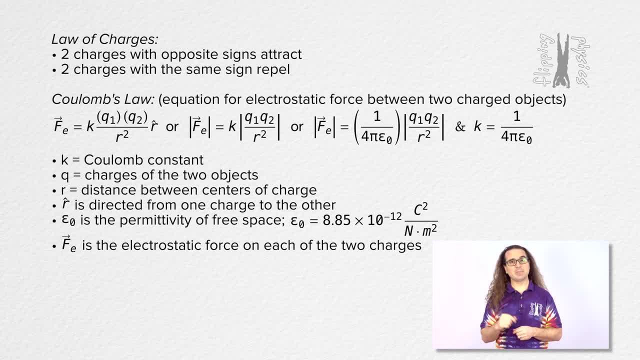 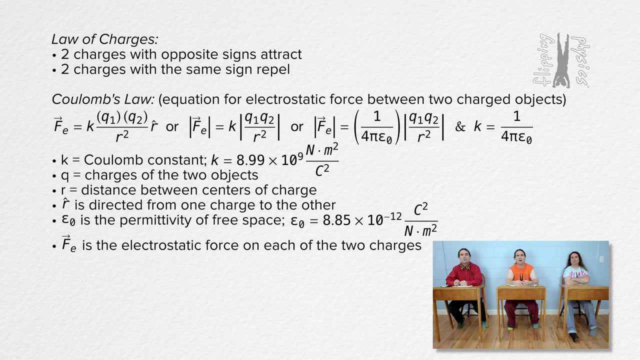 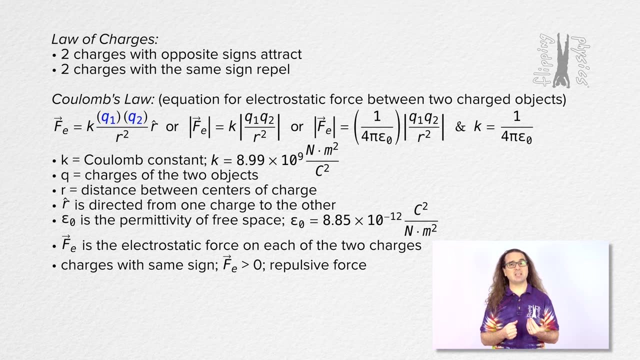 charged particles. Lowercase k is the Coulomb constant, which equals 8.99 times 10 to the ninth newtons times, meters squared over Coulomb squared. Notice that in the vector equation form of Coulomb's law, if the two charges have the same sign, the force is positive and repulsive which. 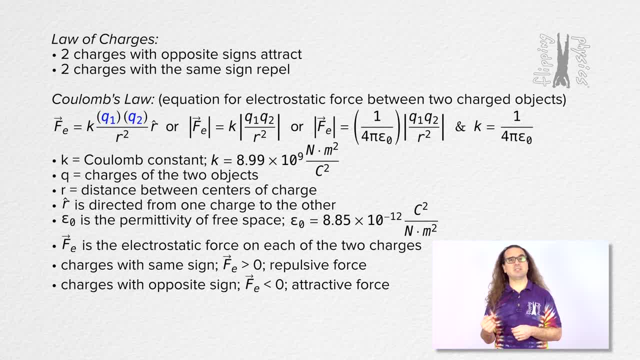 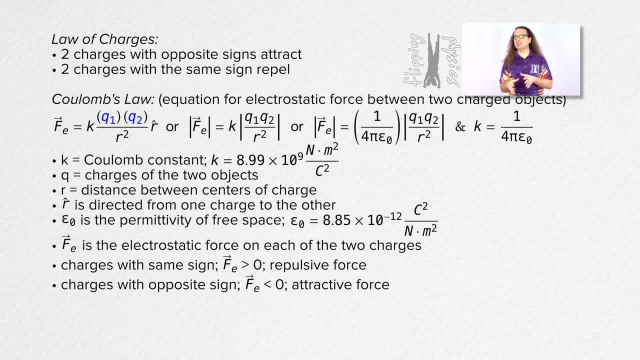 follows the law of charges And if the two charges have opposite signs, the force is negative and attractive, which again follows the law of charges. Realize this means the electrostatic force from charge 1 on charge 2 uses the unit vector from object 1 to charge 2.. 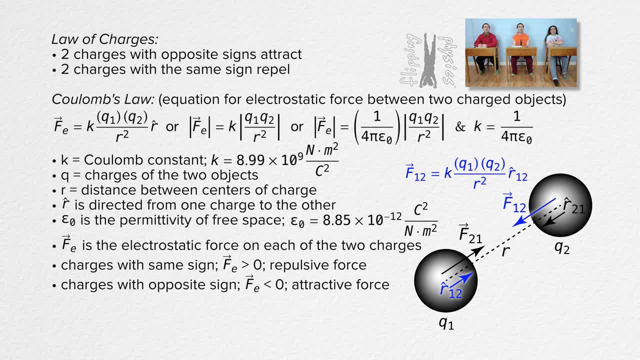 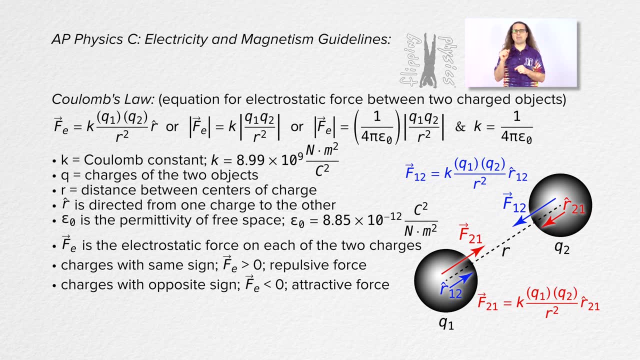 And of course, the electrostatic force from charge 2 on charge 1 uses the unit vector from charge 2 to charge 1.. Now I do want to point out that according to AP Physics C, Electricity and Magnetism guidelines, you will only be expected to calculate electrostatic forces between four. 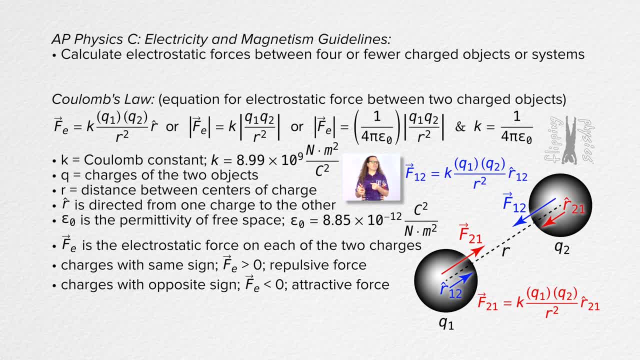 or fewer charged objects or systems. However, you may be required to analyze more than 4 charge 1 to object 2.. You can use a unit vector to calculate the unit vector from charge 2 to charge 1.. charged objects in situations which have high symmetry. So please keep that in mind. 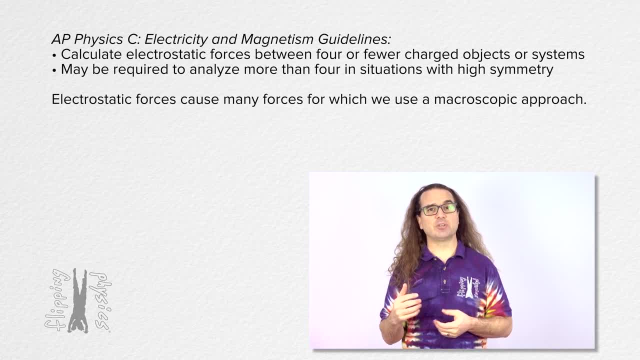 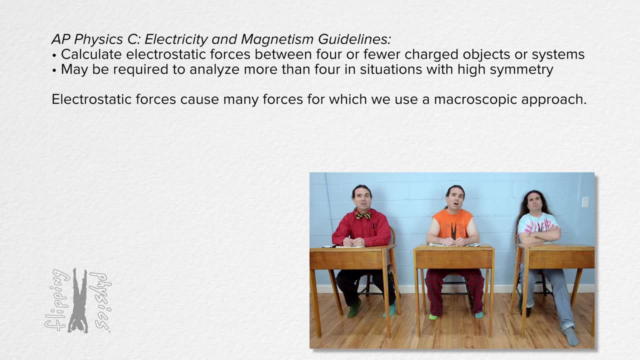 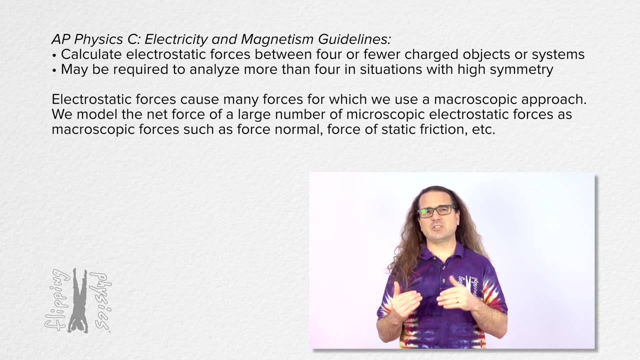 Also. the reality is that electrostatic forces, which can be determined using Coulomb's Law, cause many of the forces which we work with on a macroscopic level, For example force, normal forces of static and kinetic friction and the force of tension. There are just too many. 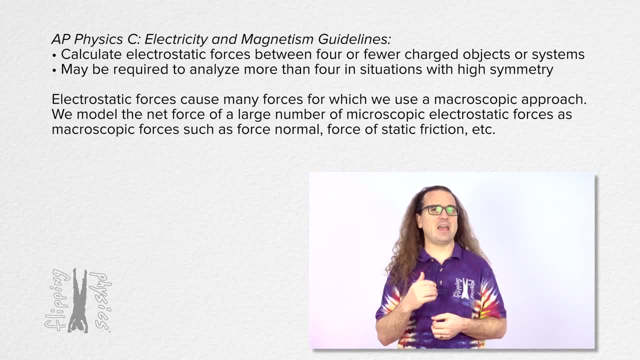 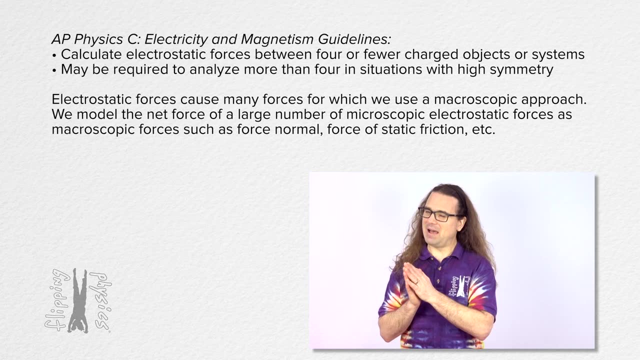 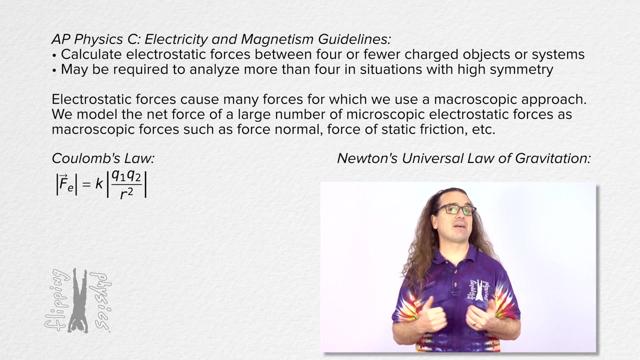 microscopic electrostatic forces to reasonably calculate every interaction, to find the macroscopic outcome. Therefore, we model the net force caused by all of these microscopic electrostatic forces as these macroscopic forces. Alright, Bobby, please discuss the similarities and differences between Coulomb's Law and Newton's Universal Law of Gravitation. 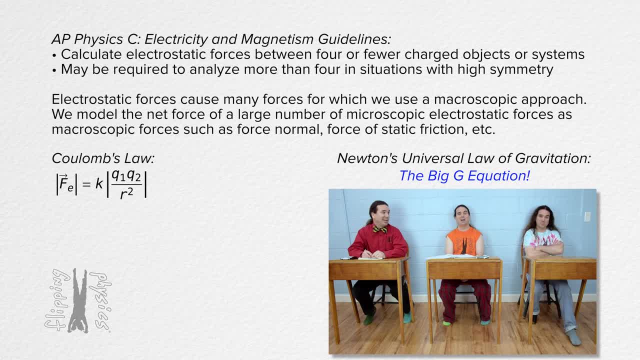 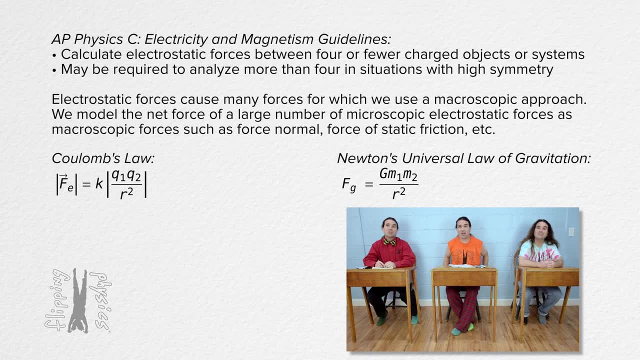 The big G equation. Yes, the big G equation, Bobby Okay Newton's Universal Law of Gravitation states that the force of gravity between two masses equals the universal gravitational constant. big G times mass 1, times mass 2,. 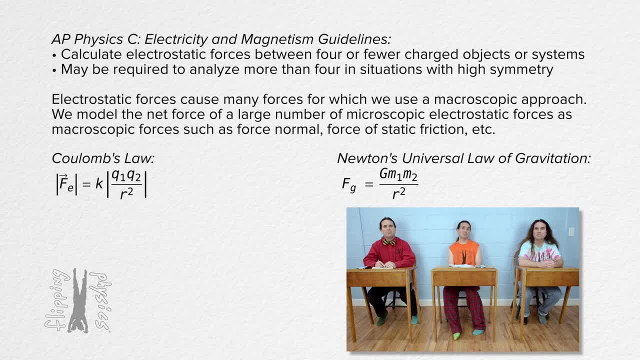 all divided by the square of r, the distance between the centers of mass of the two masses. On the AP Physics C equation sheet, it is the absolute value of the vector force of gravity. Sure, but that is the same thing as what I just said. 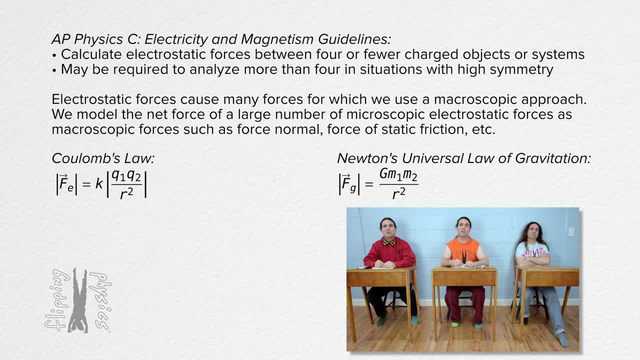 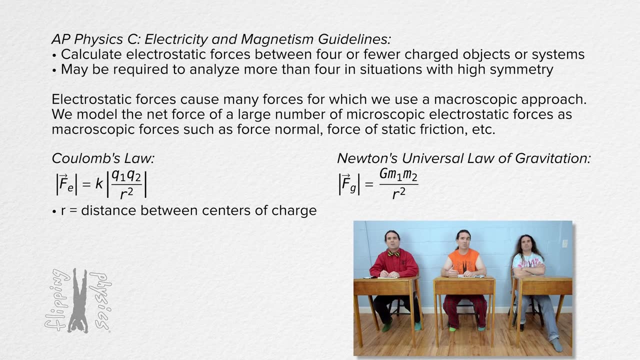 Yeah, Okay, so similarities and differences between Coulomb's Law and Newton's Universal Law of Gravitation. Well, the variable r is very similar. It is the distance between the centers of charge or the centers of mass. The electrostatic force can be attractive or repulsive. However, 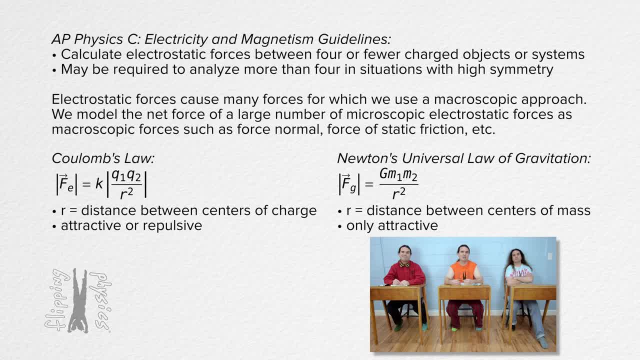 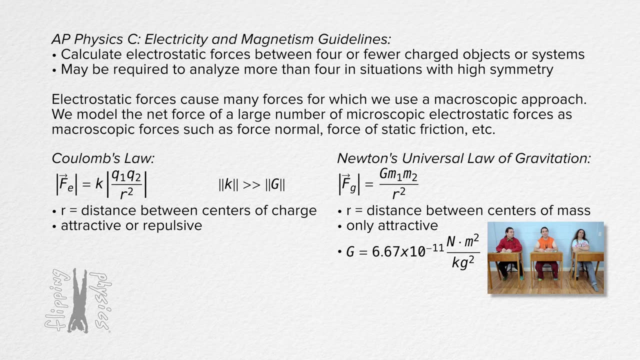 gravitational forces can only be attractive, And the Coulomb constant is much, much larger than the gravitational constant. Big G is not really that big. Yeah, Big G. the gravitational constant is only 6.67 times 10 to the negative 11 newtons times. 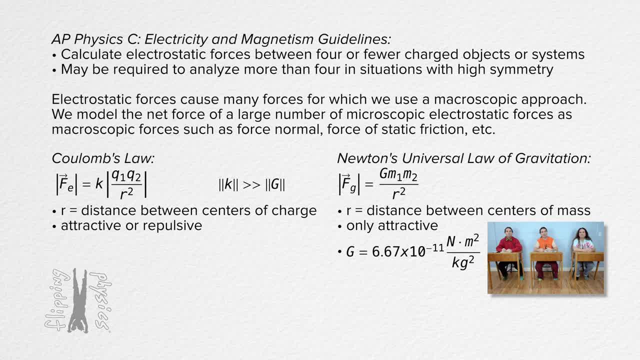 meters squared over kilograms squared, while the Coulomb constant is 8.99 times 10 to the ninth newtons times. meters squared over Coulomb squared. Yeah, The Coulomb constant is a much, much larger number than the gravitational constant. That means 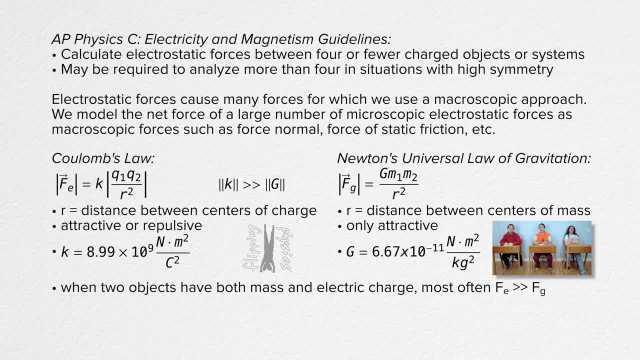 when two objects have both mass and electric charge. most often, the electric force is so much larger than the gravitational force that the gravitational force is negligible. Yeah, Poor Big G, Right Yeah. However, it is important to remember that when we are considering large-scale objects like people- planes, pineapples, planets and pre-I… Pre-I, What are pre-I …Toyota had a news conference in 2011 to announce that the preferred plural of Prius is pre-I. That is perfectly predictable. Perhaps Possibly. 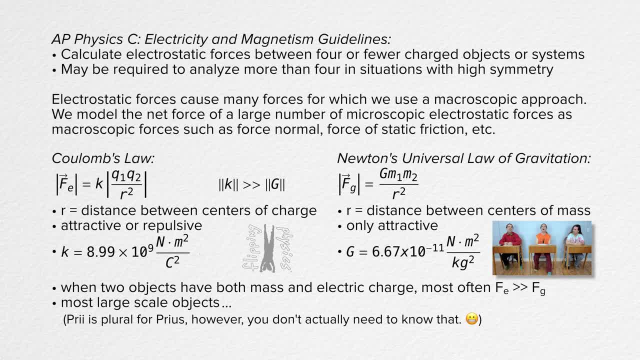 Potentially, Presumably, Probably. When we consider large-scale objects like platypuses… Or platypi …gravitational forces are large enough to make electrostatic forces negligible, because large-scale objects are usually nearly electrically neutral, In other words, 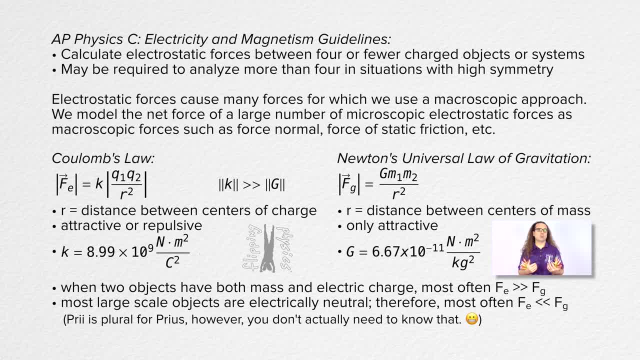 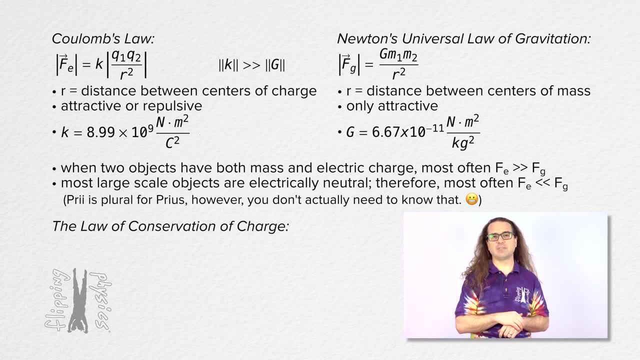 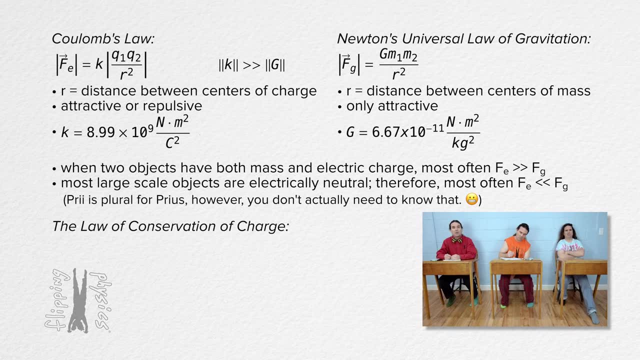 their total number of protons and electrons are nearly equal, which makes their electrostatic force small enough to be negligible. Now let's talk about the law of conservation of charge. Bo, please. The law of conservation of charge? Well, that states that the net charge of an isolated system 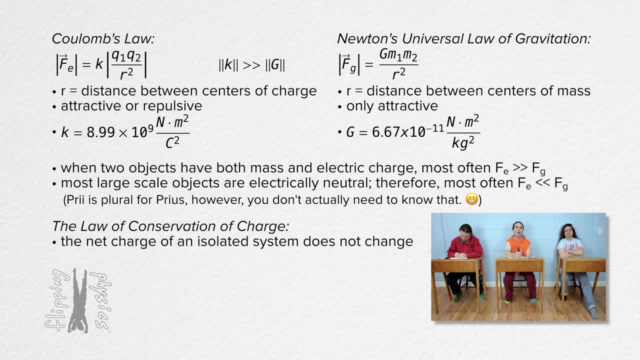 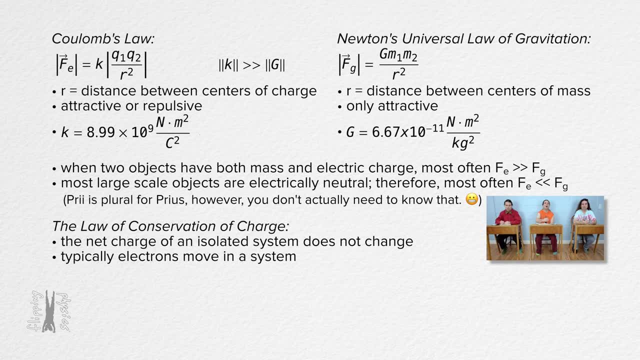 does not change. And a bit more, please. Typically, electrons are the charges which move in a system, and if there is no way for electrons to leave or enter the system- that is what makes a- a system an isolated system- then the net charge of the system will not change. 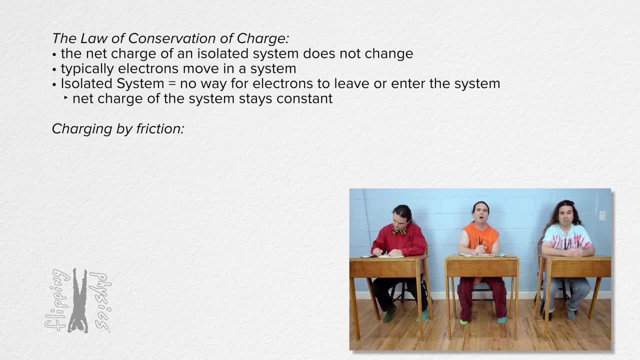 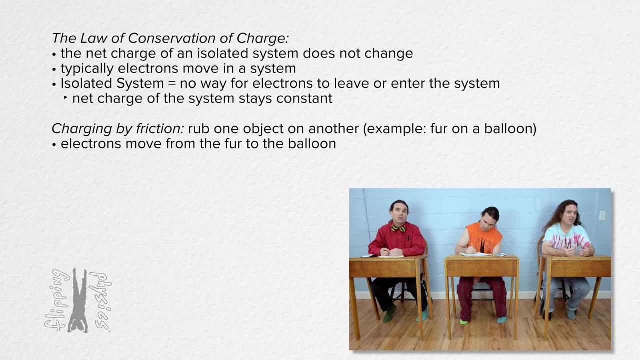 Again, please keep going. What about charging by friction? Okay, Charging by friction involves rubbing one object on another object, like fur on a balloon, for example. When this happens, electrons move from the fur to the balloon. The net charge on the balloon-fur system remains the same, because the total number of protons and electrons in 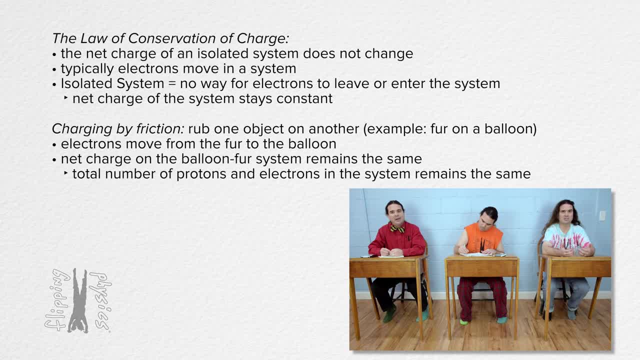 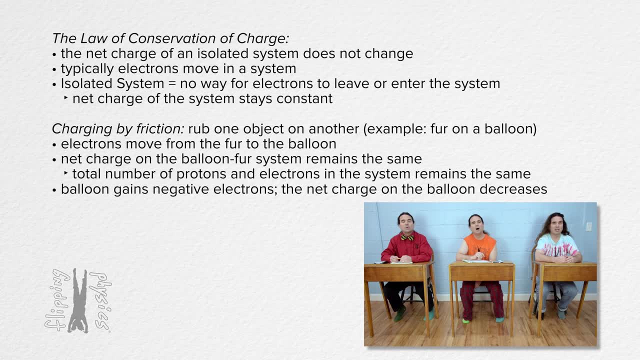 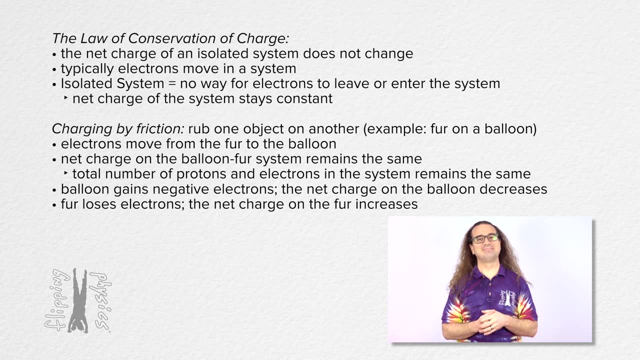 the system remains the same, but you know, the two objects in the system have had their net charge change. The balloon gains negative electrons, making the net charge on the balloon more negative. The fur loses electrons, making the net charge on the fur more positive. 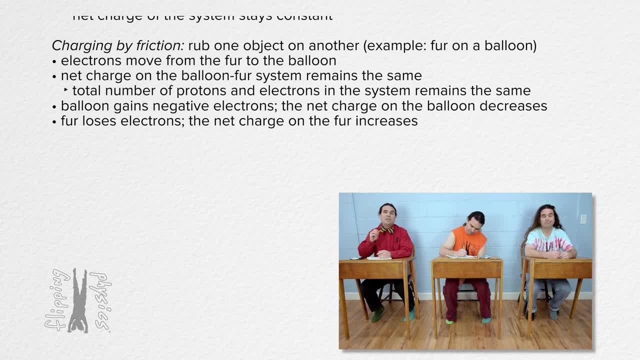 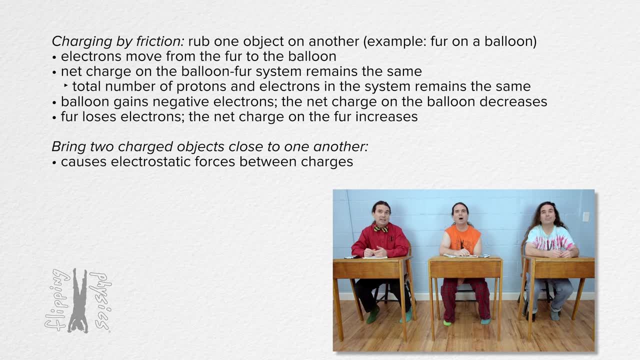 That is charging by friction, And when you bring two charged electrons into the balloon the net charge on the balloon becomes negative. When you bring two charged objects close to one another, that will cause electrostatic forces between the charges and can change the distribution of the electrons in the objects. This can 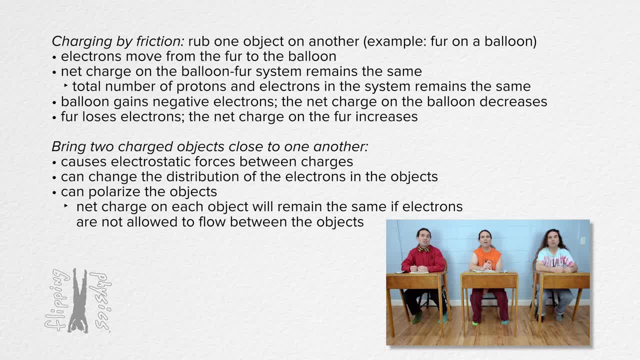 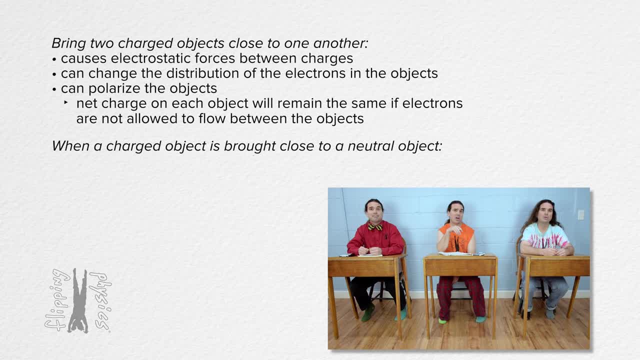 polarize the objects, however, the net charge on each object will remain the same if electrons are not allowed to flow between the objects. When a charged object is brought close to a neutral object, the charged object can rearrange the charges in the neutral object and cause a charge. 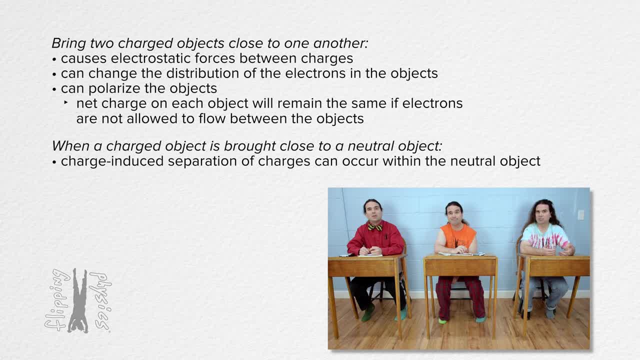 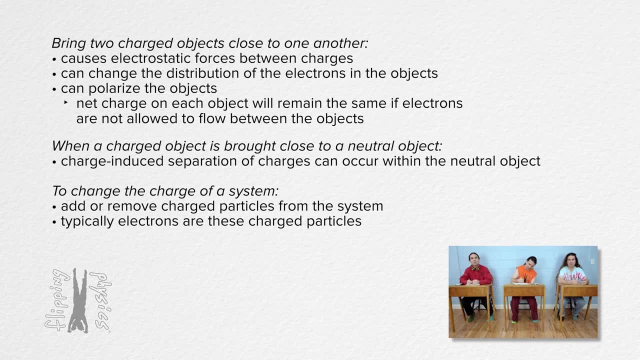 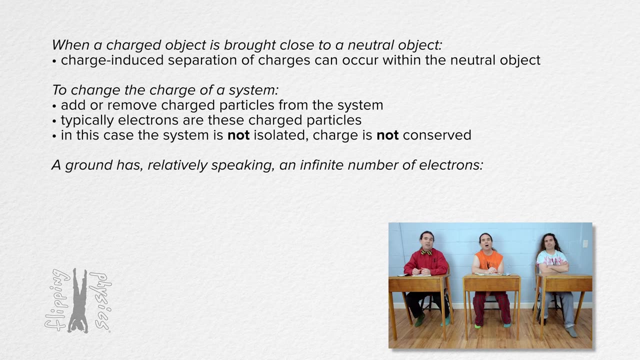 induced separation of charges in the neutral object. Most often, the way to change the charge of a system is to add or remove electrons from the system. When that happens, the system is not isolated and the charge is not conserved. Oh, and we should talk about grounding. A ground has, relatively speaking, 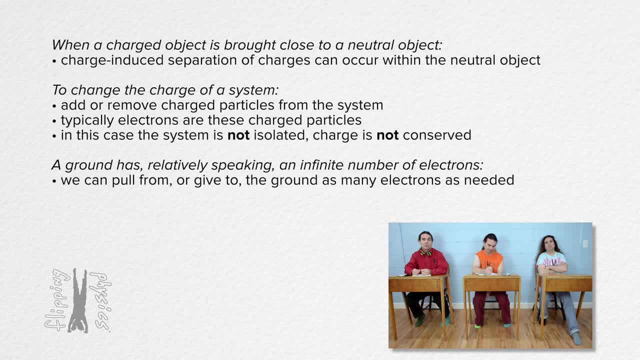 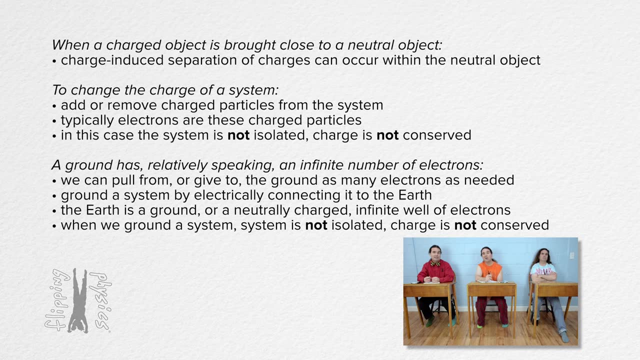 an infinite number of electrons which we can pull from it or we can give to it. We can ground a system by electrically connecting it to the earth, which is which is a ground or a neutrally charged infinite well of electrons. When we ground a system, the system is not isolated and charge is not conserved. 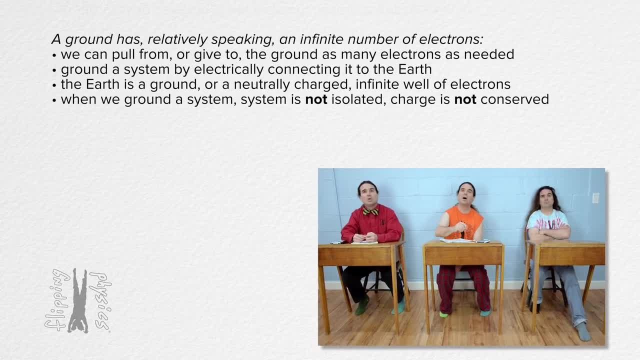 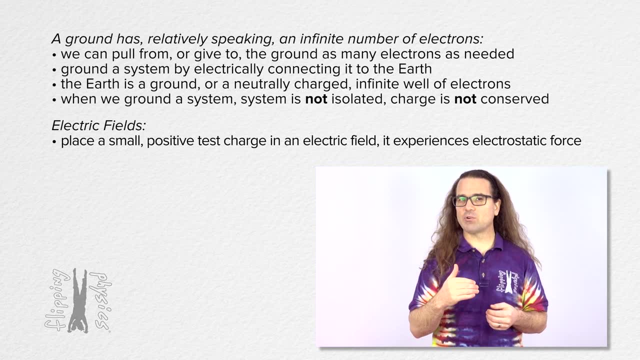 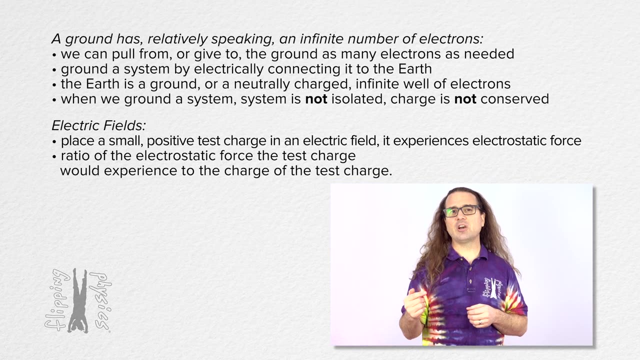 Very nice everybody. Now we need to talk about electric fields. If we were to place a small positive test charge in an electric field, it would experience an electrostatic force caused by the interaction of the small positive test charge with the electric field. An electric field is the ratio of the electrostatic force the small. 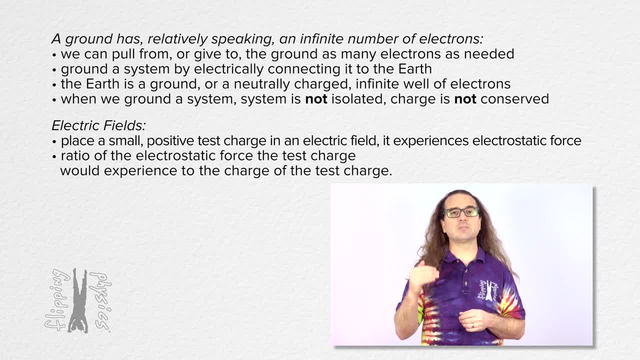 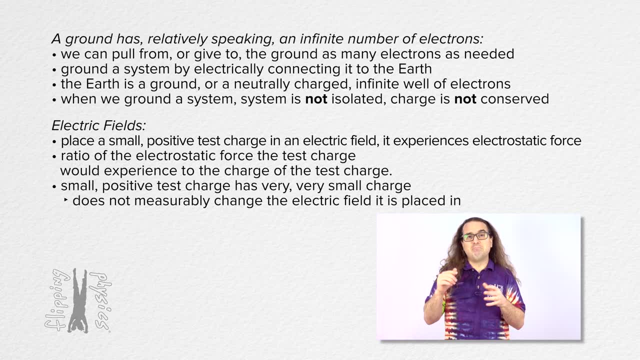 positive test charge would experience to the charge of the small positive test charge. A small positive test charge is a charge which is small enough not to measurably change the electric field it is placed in The equation for an electric field is electric field equals. 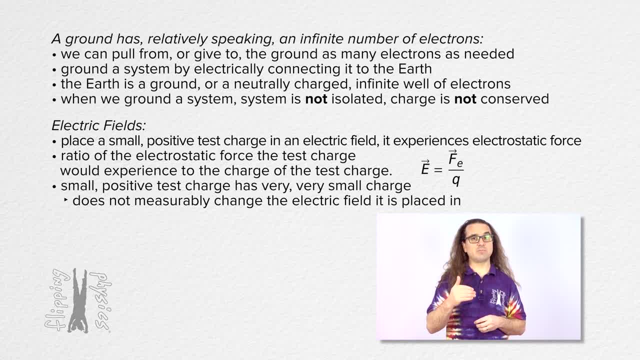 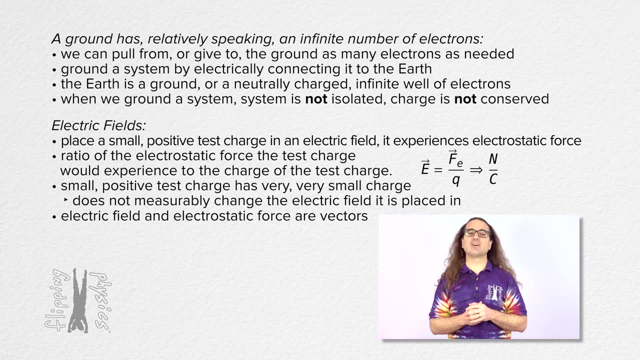 electrostatic force divided by the charge of the small positive test charge, where both electric field and electrostatic force are vectors. Notice this means the units on the electric field are per coulomb and please realize electric field is a vector, Therefore class, it has both. 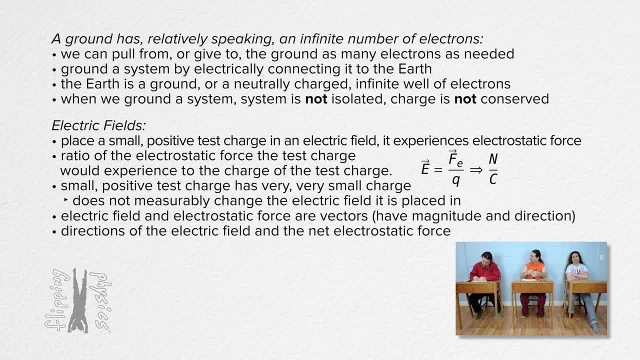 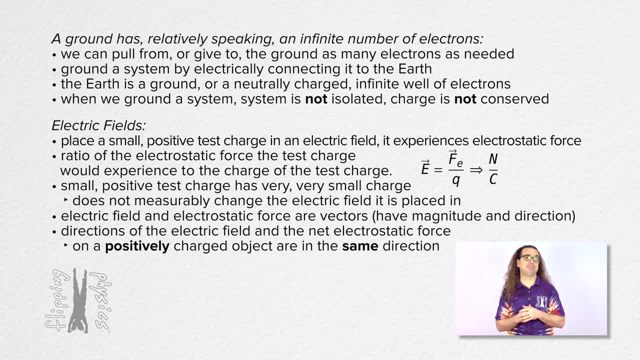 magnitude and direction. Notice: the electric field and the electrostatic force experienced by a positive charge in an electric field will be in the same direction, Because electric field and electrostatic forces are both vectors in that equation and therefore they have to be in the same direction Exactly. 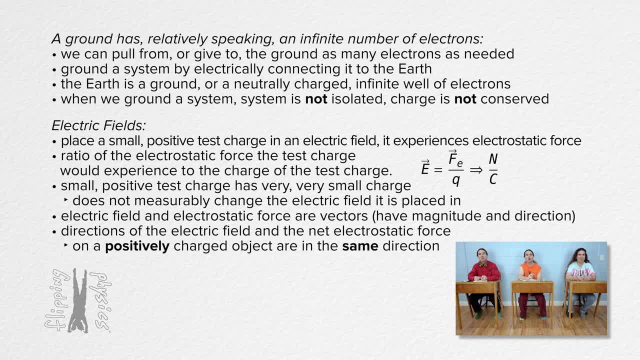 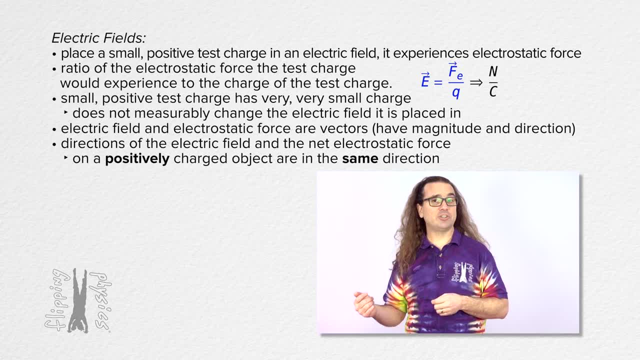 Hold up. What if the charge we put in the electric field is negative? I don't think the vectors will be in the same direction then. Good point, Bo. Looking at the equation, how do you think using a negative charge changes the direction of the force experienced by the? 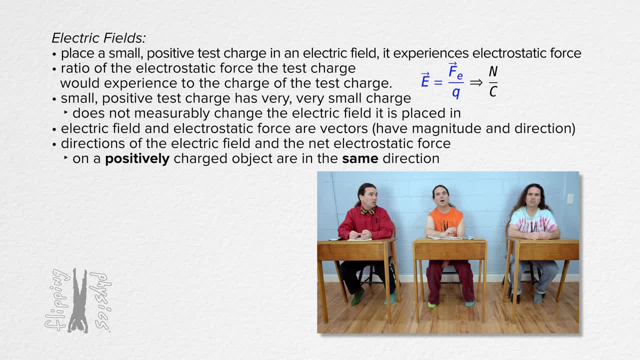 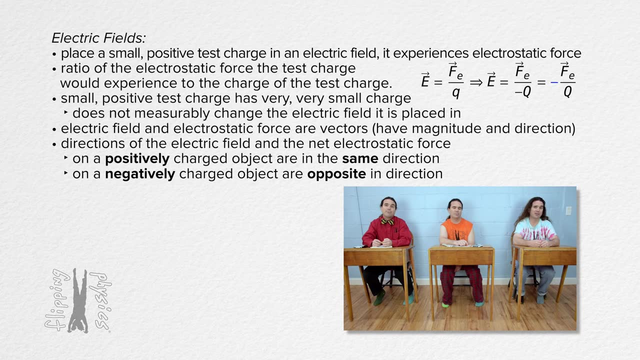 charge. Um, When the charge is negative in the equation. Oh, I see. Okay, That makes the force experienced by the negative charge and the direction of the electric field opposite in direction because of the negative in the equation. That totally works. 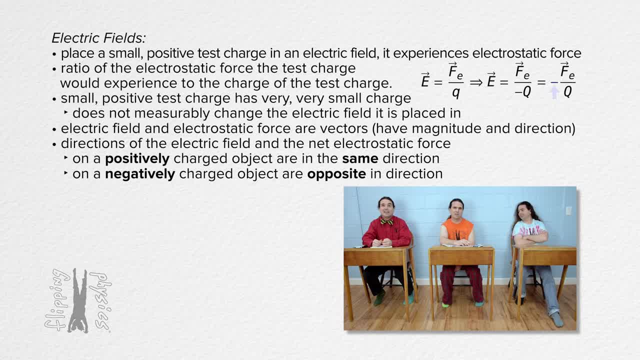 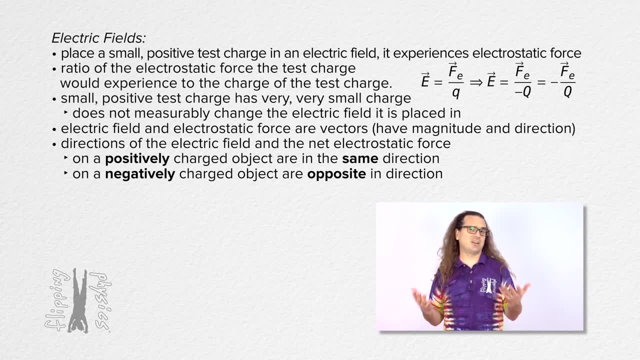 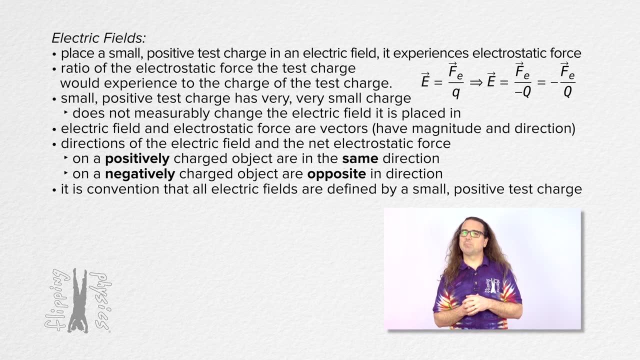 Sure, But why do we always use a positive test charge and not a negative test charge? The reason we use a positive test charge is just convention. That is how all electric fields are defined, using a positive test charge. Okay, Bobby, please tell me what the 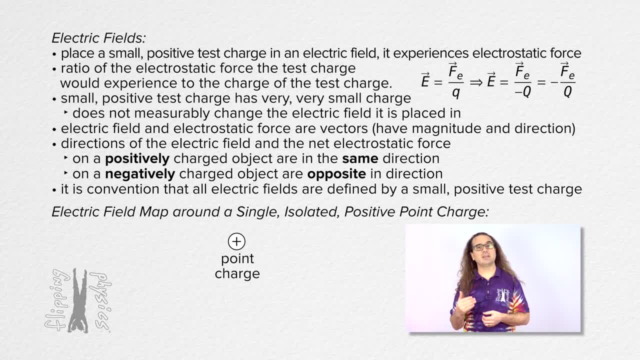 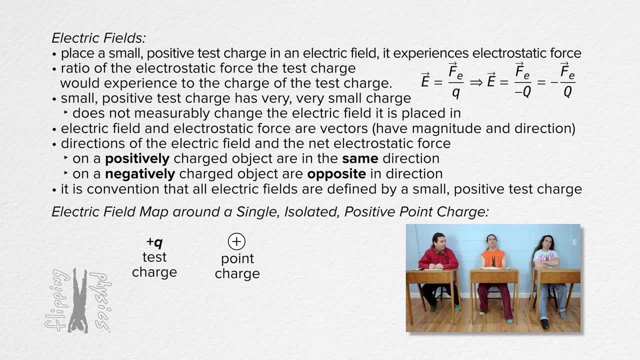 electric field map looks like around a single isolated positive point charge. When we take a positive test charge and place it near the positive point charge, according to the law of charges, because both charges are positive and therefore have the same sign, the positive test charge will be repelled from the positive point charge. That means no. 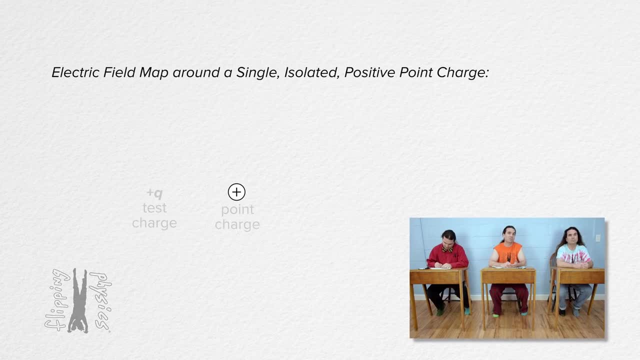 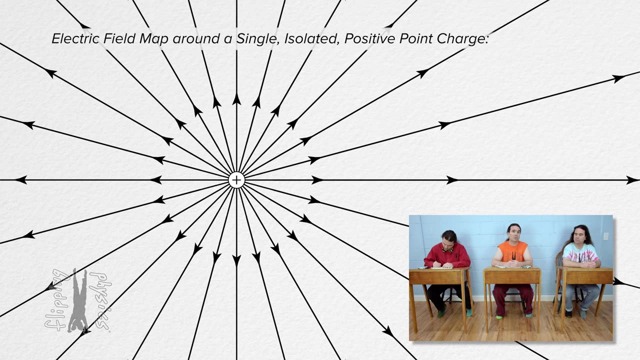 matter where we place the positive test charge, it will experience an electrostatic force radially outward from the positive point charge. Also, we know that, according to Coulomb's law, the magnitude of the force will decrease as the positive test charge gets farther from the 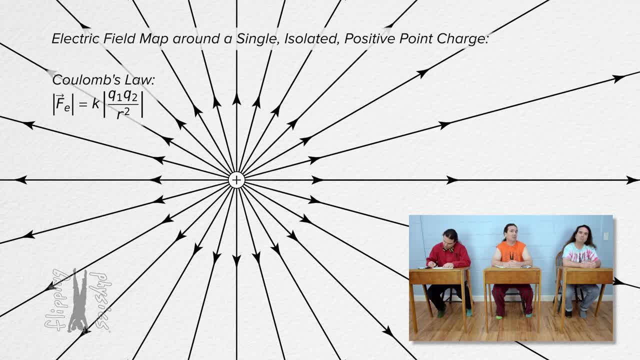 positive point charge. So the positive test charge will be repelled from the positive point charge. Therefore the electric field which surrounds a positive point charge is always directed outward, away from the positive point charge and decreases in magnitude as we get further from the positive point charge. We can determine the equation for that electric field by plugging. 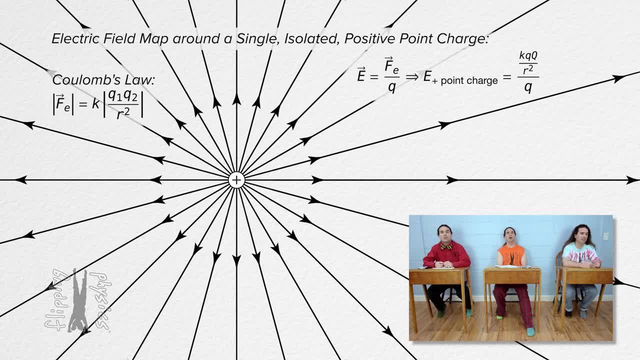 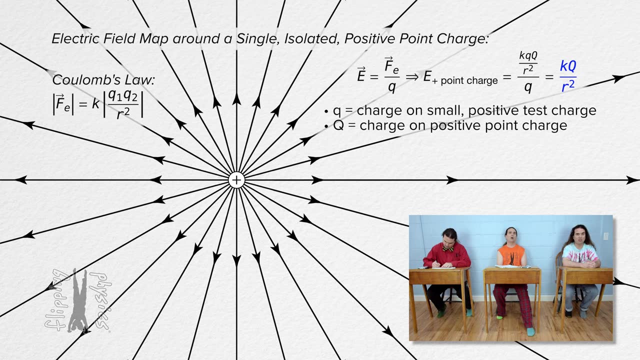 the electrostatic force equation into the electric field equation. Using q for the positive test charge and q for the positive point charge, we get that the electric field which surrounds the positive point charge equals the Coulomb constant times the point charge all over the square of r, which is the distance between centers of charge. Actually, no, r is the distance from. 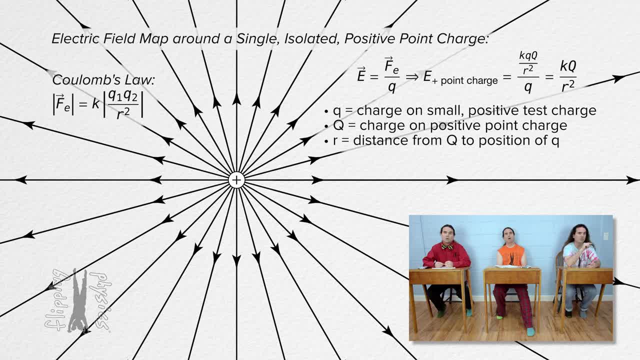 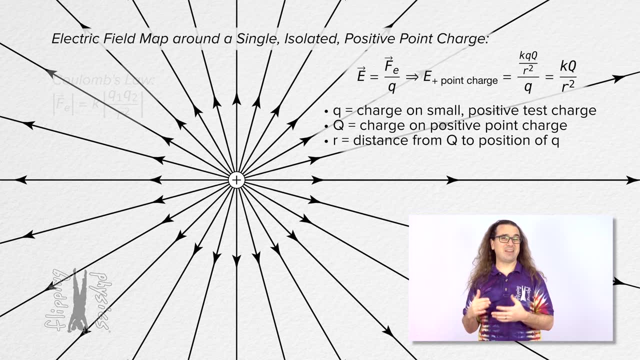 the center of the positive point charge to the location of the positive test charge or the location we are defining the electric field. That equation matches the diagram Bobby drew right. Mr B, Absolutely, Bo And Bo. what does the electric field around a negative point charge? 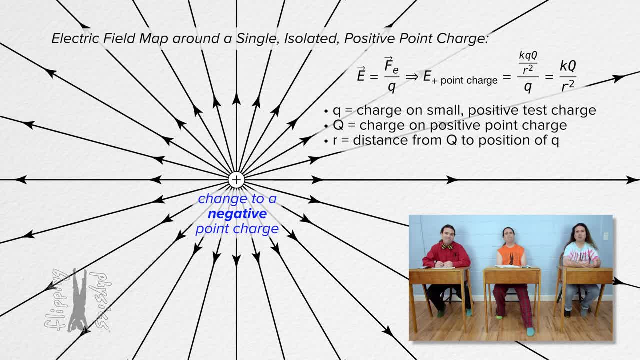 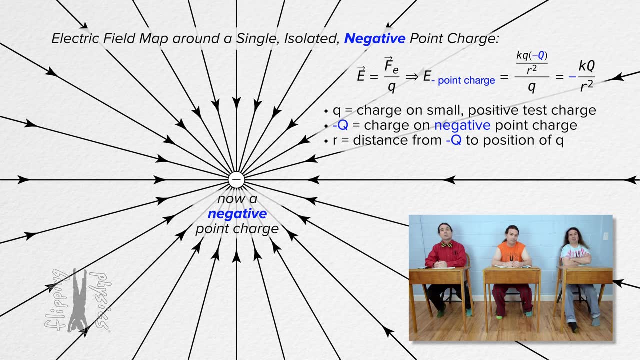 look like. Well, it ends up being the same equation, only capital Q, the charge of the point charge is negative. That means all the field lines go toward the negative point charge. It's almost the same as for the positive point charge, only all the arrows point radially inward toward. 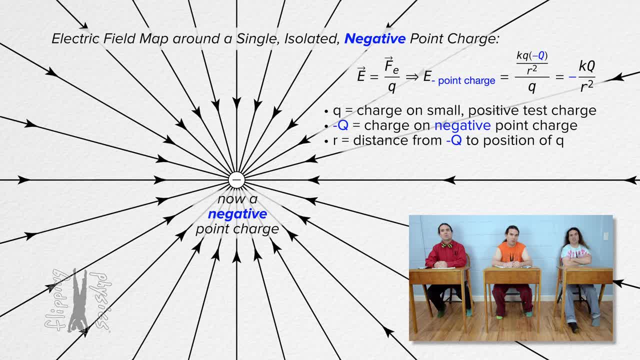 the negative point charge because the law of charges says the positive test charge will be attracted to the negative point charge because the two have opposite charge signs. Correct, Bo. thanks Now, Mr P. Yes, Bobby, That looks a lot like the gravitational field which exists around a planet, right? 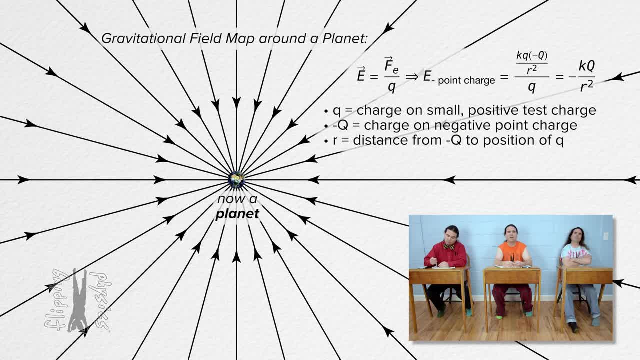 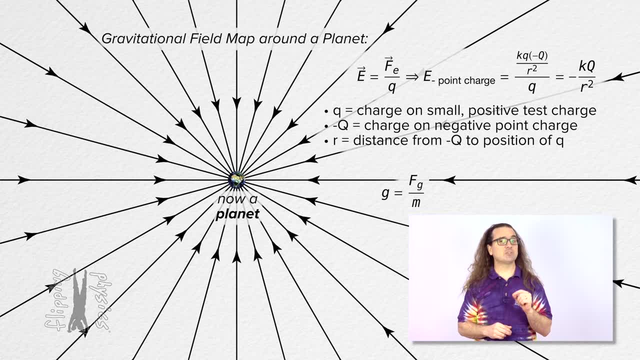 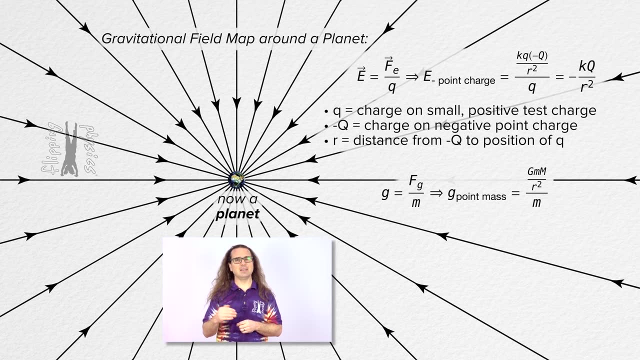 Yes, Bobby, that is correct. Why is that? That is a fair question, Bobby. Remember that the gravitational field equals the force of gravity divided by the mass of a small test mass, And we can substitute Newton's universal law of gravitation in for the force of gravity. 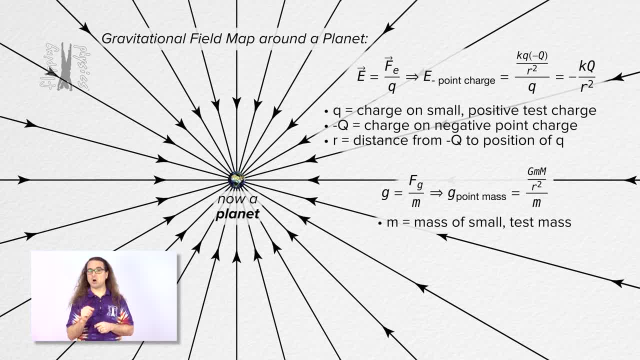 Using lower case m for the mass of the small test mass and upper case m for the mass of the point mass. And we get that the gravitational field around a point mass equals the gravitational constant times the mass of the point mass divided by the square of r. 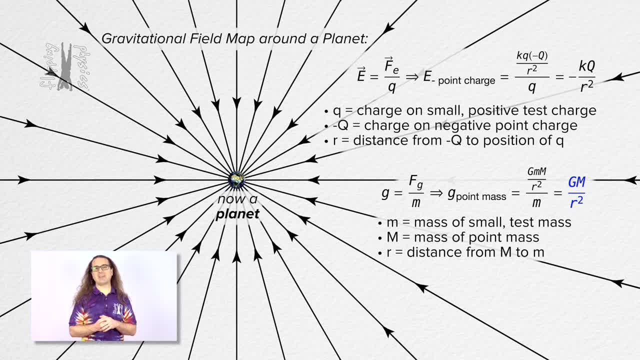 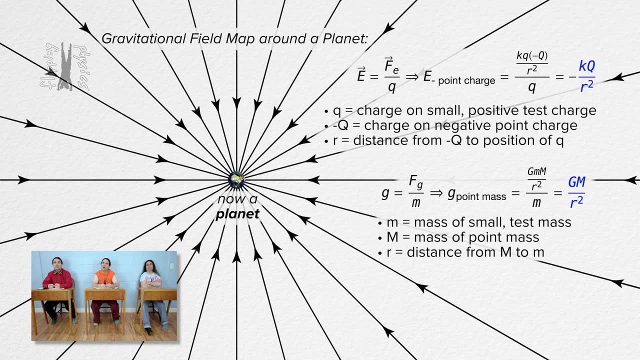 the distance from the center of the point mass to the location of the small test mass or the location the gravitational field, And that equation is similar to the equation for the electric field around a point charge, which is why the gravitational field around a planet and the electric field around a negative 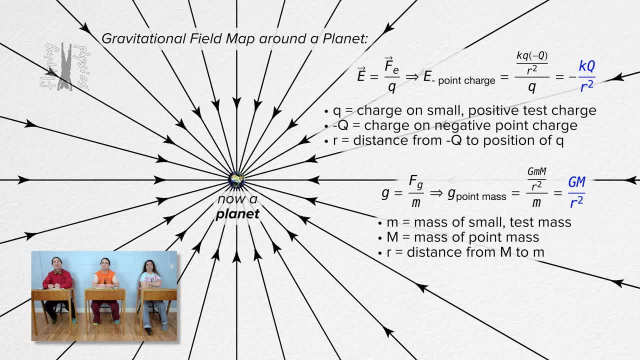 point charge. look the same. How come we can treat a planet as a point mass? When we get far enough away from a planet, we can treat a planet as a point mass like we do here. Sure, but have we ever been that far from Earth? 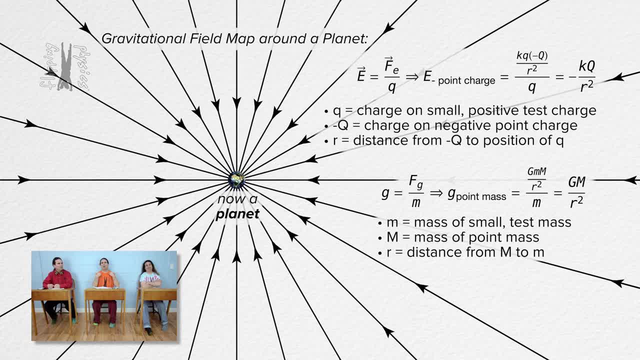 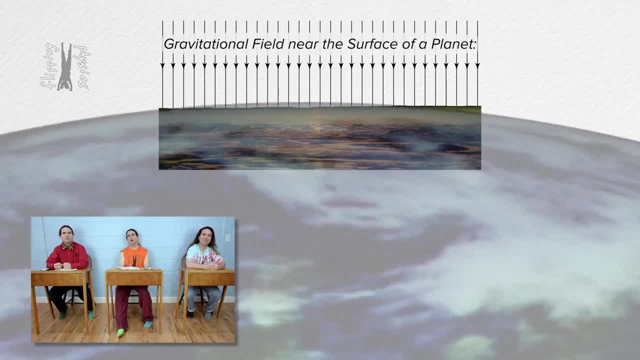 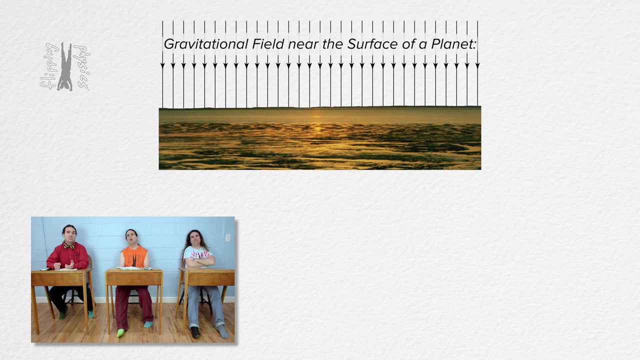 Depends on how you define we. Uh, if you are actually standing on the surface of a planet, like we are currently on planet Earth, we can consider the gravitational field to be constant and pointed down toward the Earth, and that looks just like the electric field that exists between two large parallel. 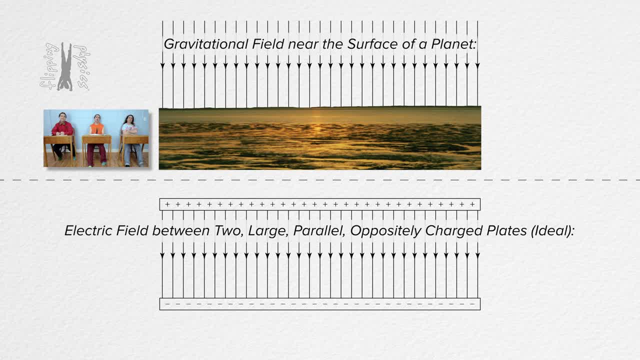 oppositely charged plates. Right, Mr P? That is a valid point, Billy, But please remember that is for an ideal case Where the two parallel plates are very large relative to the space between the two plates. In a non-ideal case, the two parallel plates will have an electric field which curves a. 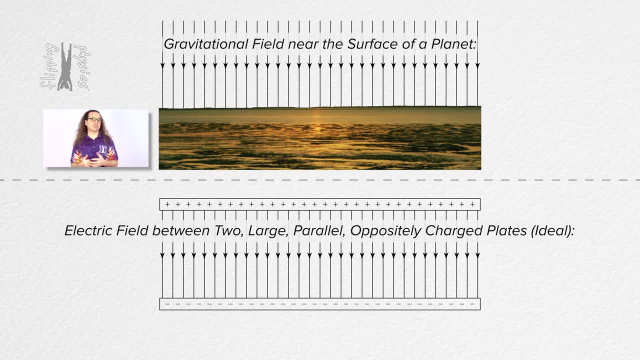 bit near the edges of the plates and there will be some electric field which exists outside the parallel plates. Billy, let's walk through one more electric field map. Please tell me what the electric field map for two point charges, one positive and one negative, which are isolated from all other points. 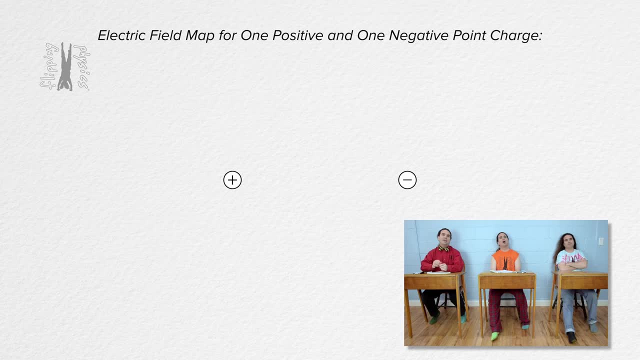 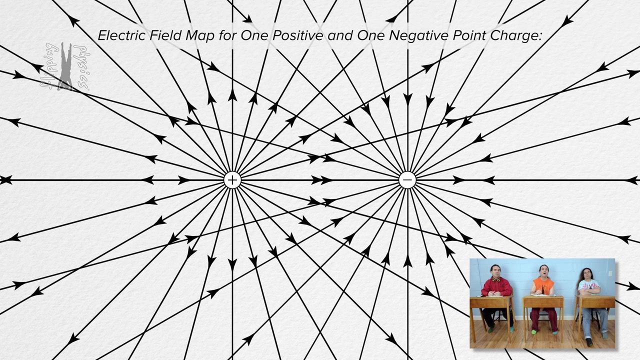 Okay, A positive and negative point charge are isolated from all other charges. We already know what the electric fields which surround a single positive point charge and a single negative point charge look like, So let's add those electric fields for each of the charges. 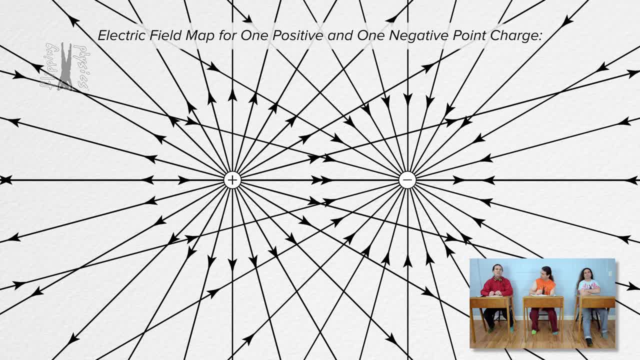 Actually that's kind of confusing. So let's make the electric field from the positive charge blue and the electric field from the negative charge red. Okay, Because the electric field is a vector, the electric field from both point charges will be the sum of the electric fields for both charges. 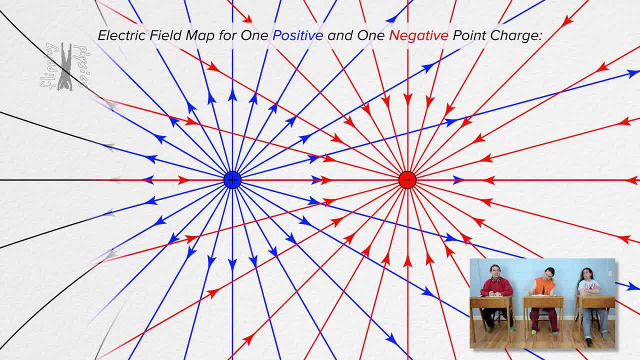 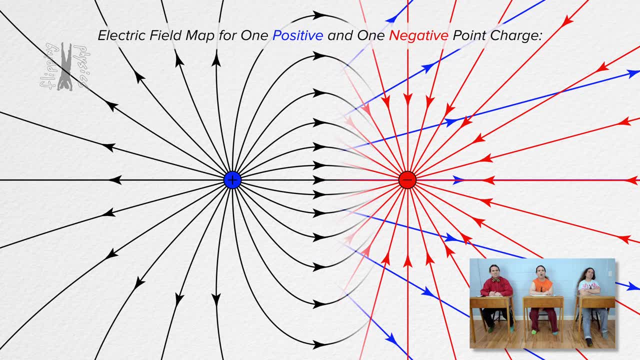 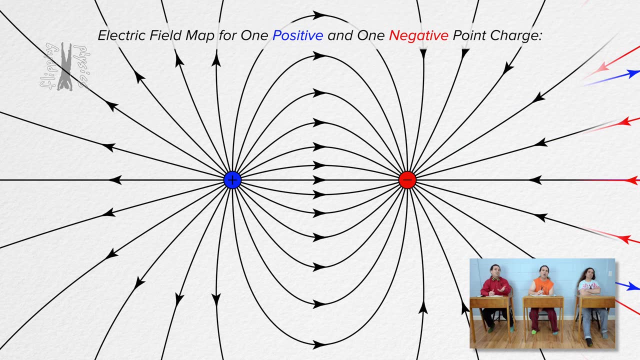 That means we need to do vector addition of each of those electric fields So we can go through and approximate the vector addition of both electric fields And we end up with a net electric field which looks like it does in the net electric field map you are showing there in black. 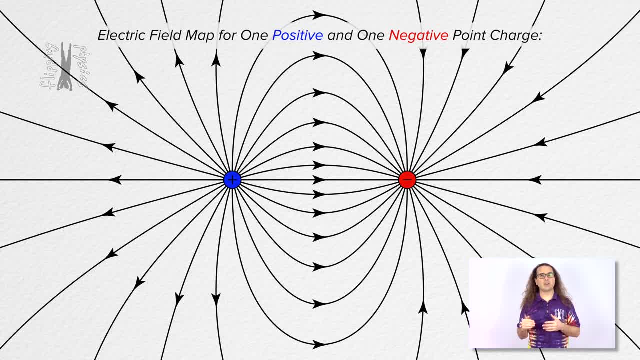 Thank you, Billy. Please realize electric field maps like this one are simplified models and are vector field maps which show the magnitude and direction of the electric field for an entire region. You know what? We never actually went over the basics of electric field lines. 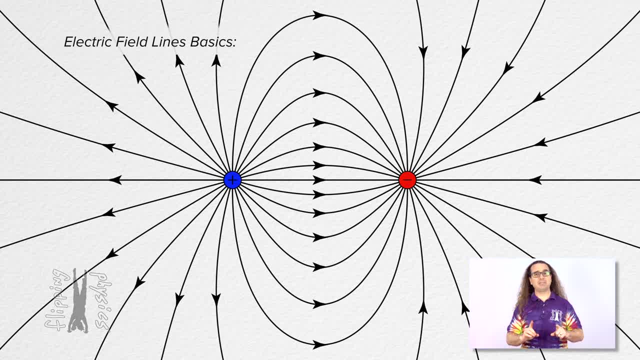 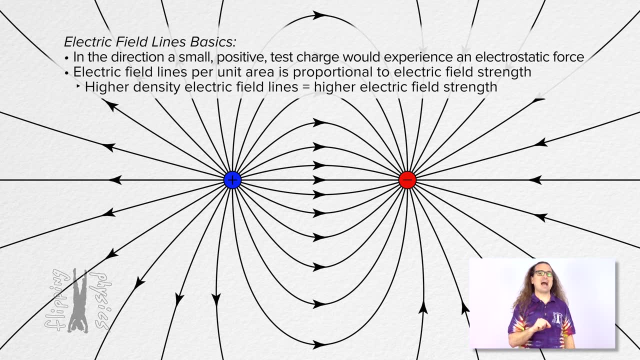 I think we should do that. Yeah, Okay, Electric field lines are always in the direction. a small positive test charge would experience an electrostatic force. The number of electric field lines per unit area is proportional to electric field strength. In other words, a higher density of electric field lines means a higher electric field. 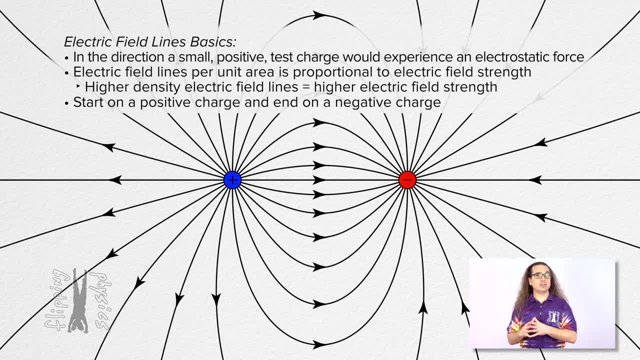 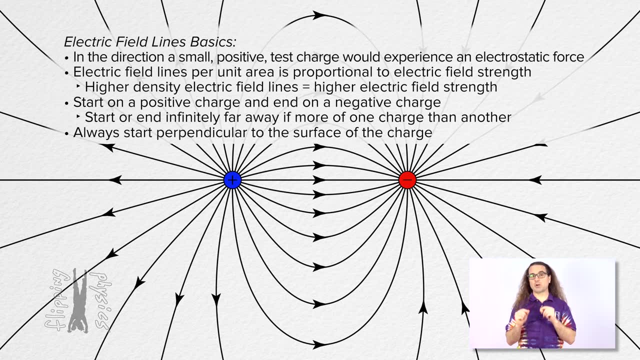 strength. Electric field lines always start on a positive charge and end on a negative charge. unless there is more of one charge than the other, then some of the electric field lines end or start infinitely far away. Electric field lines always start perpendicular to the surface of the charged objects. 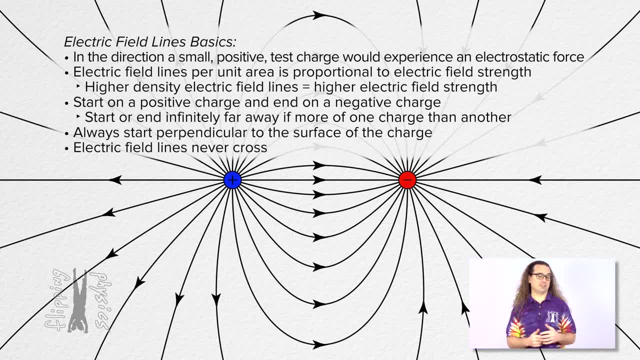 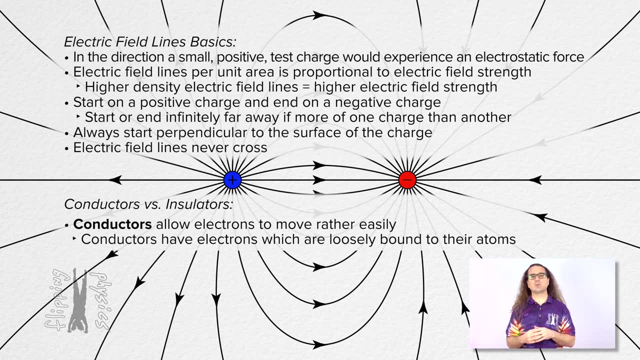 And lastly, electric field lines will never cross. Okay, Now let's talk about conductors versus insulators. Conductors are materials which allow electrons to move rather easily. This is because conductors have electrons which are loosely bound to their atoms, which